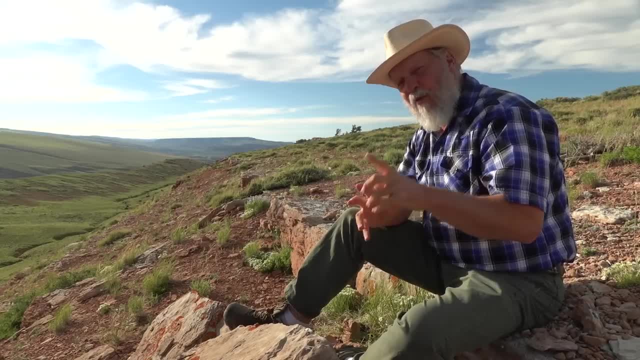 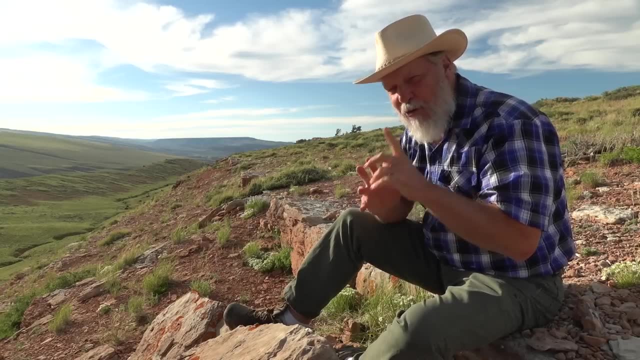 Because we can determine that. Now many of you will say, well, I know how that's done. That's using radiometric dating with radioactive isotopes of elements, And you're right, but there's a lot more to it and it's far more interesting. in my humble 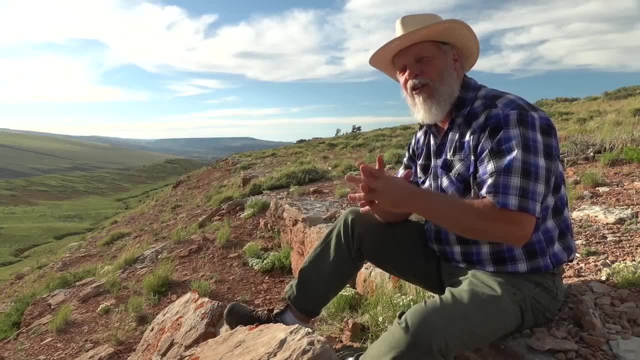 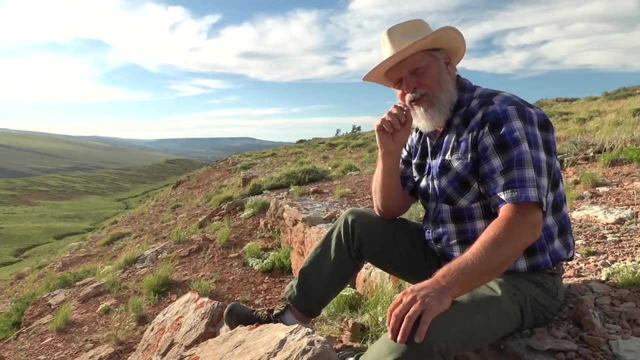 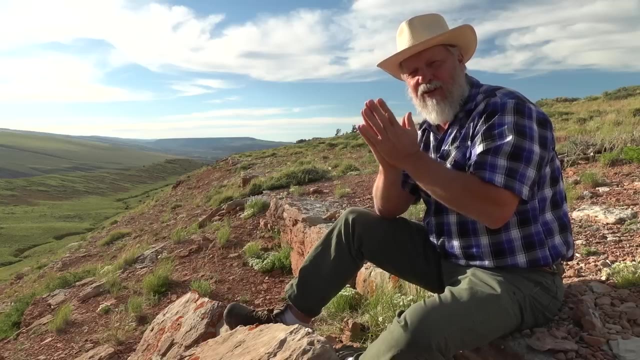 opinion where we get into some basic geology that I think you'll follow really well. this video is not about radiometric dating, although I'll mention it just a little and we'll touch that subject, but it's. but it's how to use basic geology principle, geological principles to date, when these 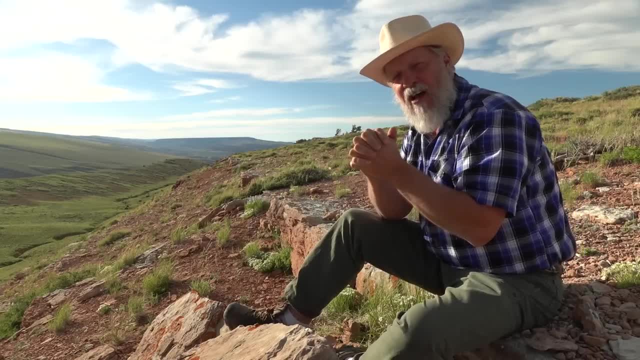 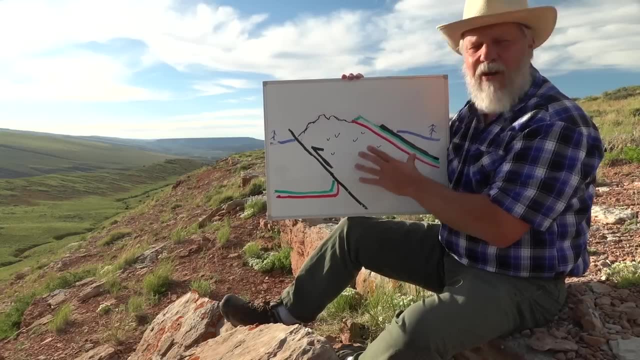 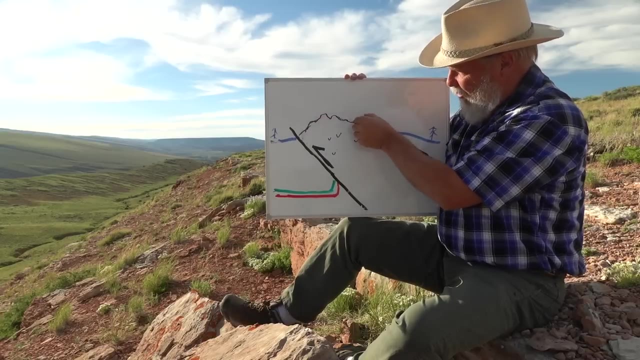 spectacular mountains like these Wind River Mountains are uplifted. have our how long it took them to occur. with my whiteboard here, I want to show you a sketch of the Wind River Mountains. so this this represents the Wind River Mountains right here and these are the layers of rock. I've just put a couple. 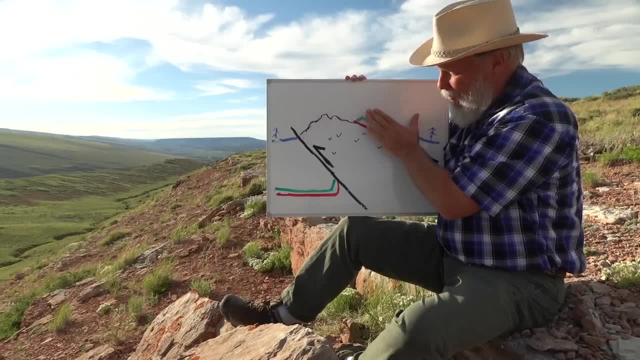 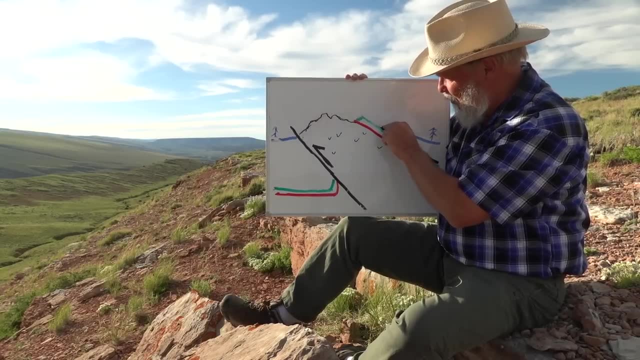 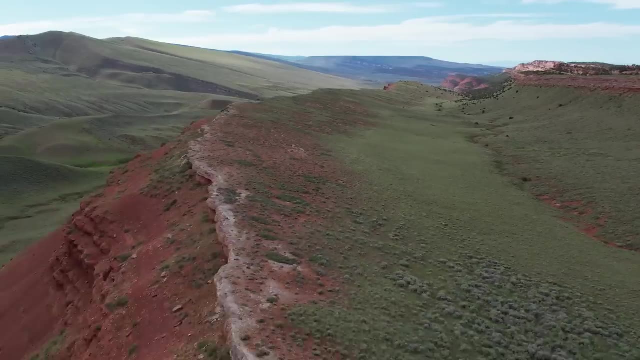 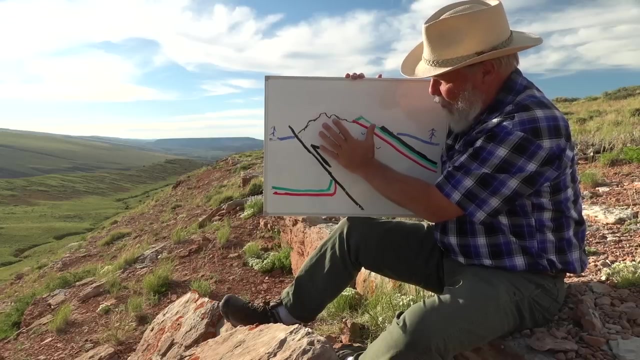 diagrammatically here on the flank of the Wind River Mountain. okay, here we're standing cartoon wise, right here, or I'm sitting right here here on a great, huge, thick formation called the Chugwater Formation. It's 250 million years old, spectacular red beds that we're kind of familiar with now. This is the core. 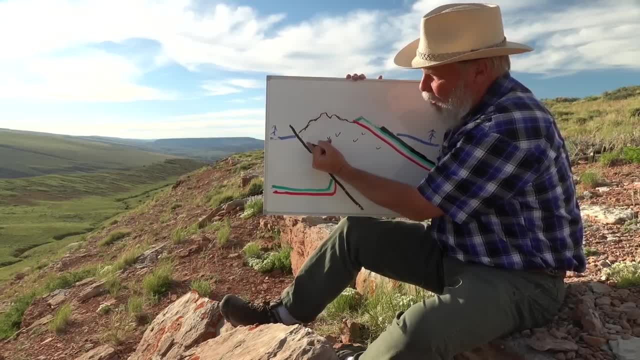 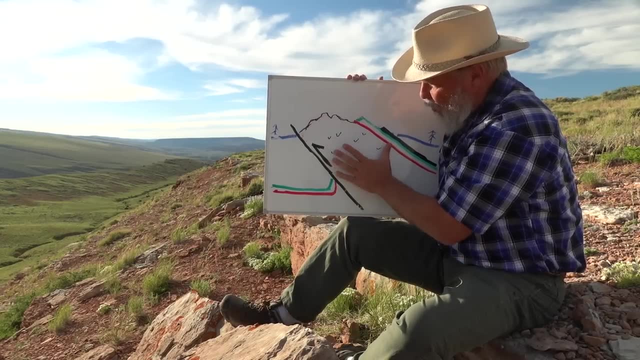 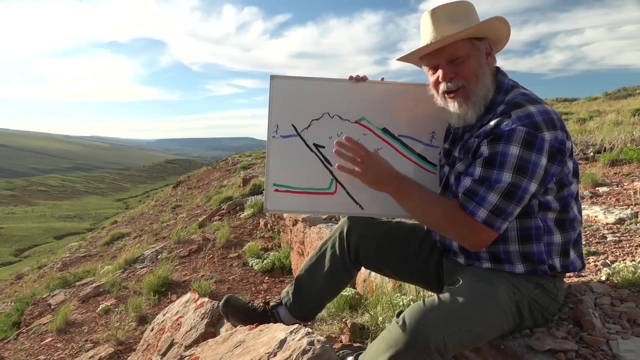 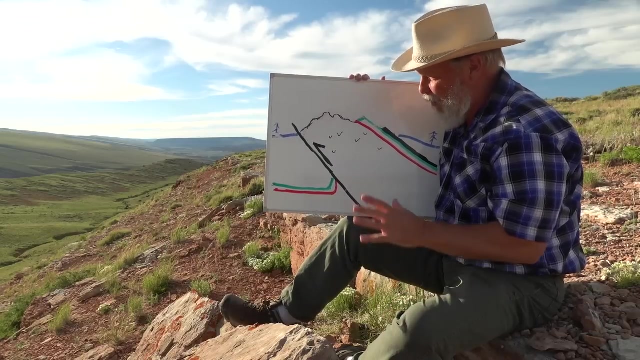 This is basement rock. This is a gigantic fault, huge back thrust, thrust fault. This arrow shows the direction. here, This mountain, this core, the basement rock, came up along this fault. This fault is unbelievable. It was uplifted 30,000, over 30,000 feet, Unbelievable. 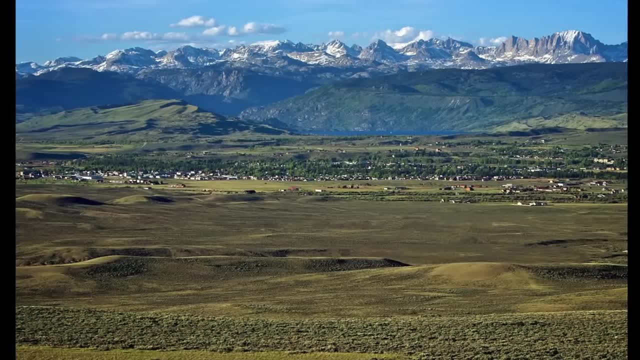 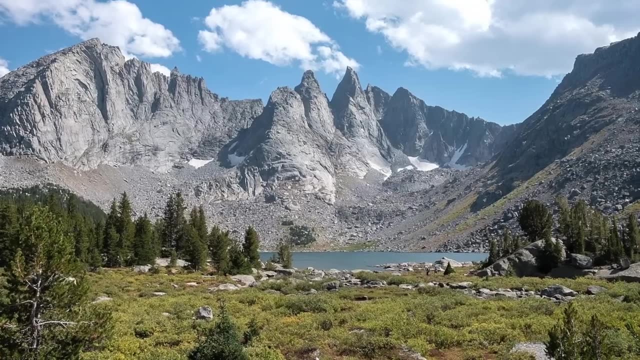 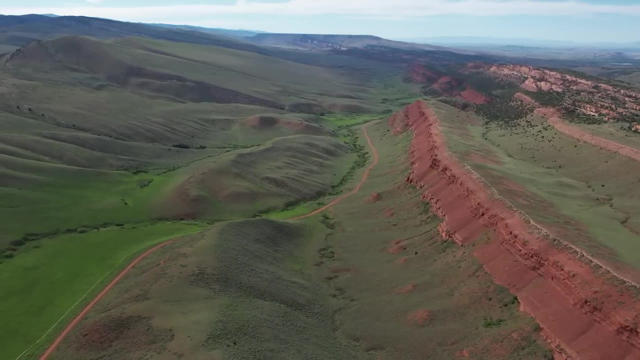 to bring all this mountain up. Geologists have determined that the Wind River Mountains started uplifting about 65 million years ago and finish uplifting 15 million years later. It turns out that these spectacular formations are the result of a great, huge, thick formation called the Chugwater Formation. 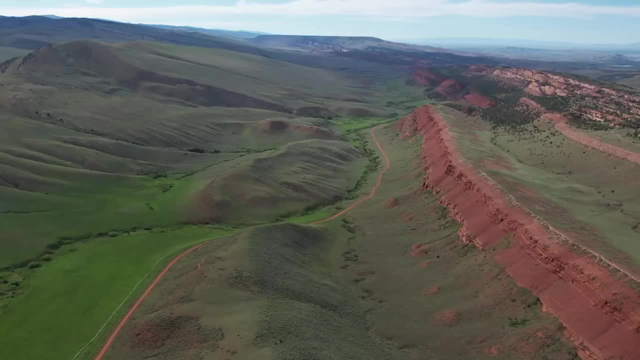 It's 250 million years old spectacular red beds that we're kind of familiar with. now. This is a great, huge, thick formation. It's 250 million years old spectacular wood. These formations of sloping rocks we see on the sides of so many mountain ranges tell 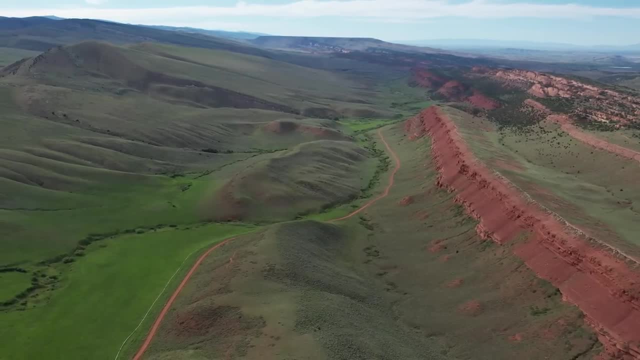 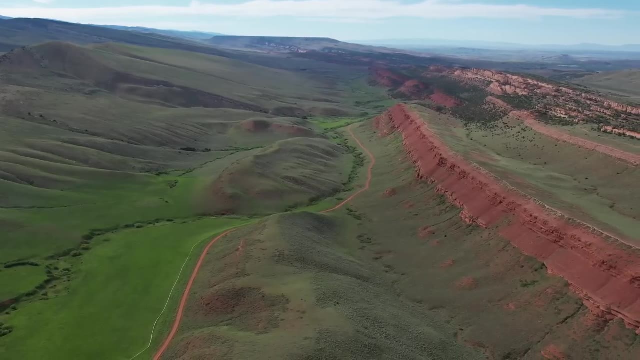 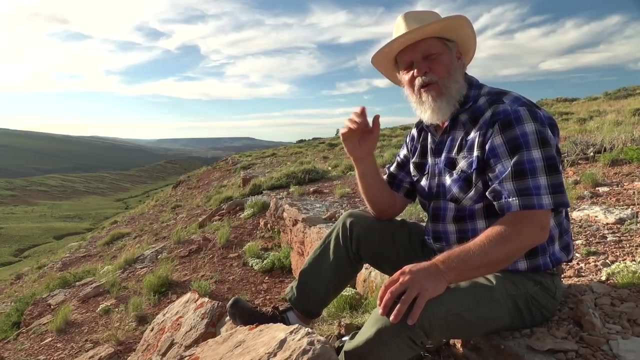 us the story of when the mountain was uplifted. All we need to do is to understand a few basic geological principles to reveal this amazing history. So let's move on on this great field trip to the Bighorn Basin back in my home country. 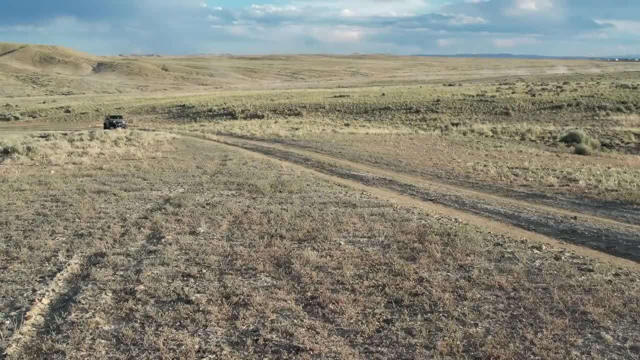 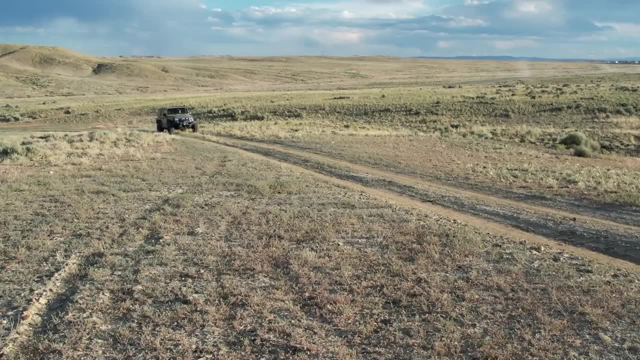 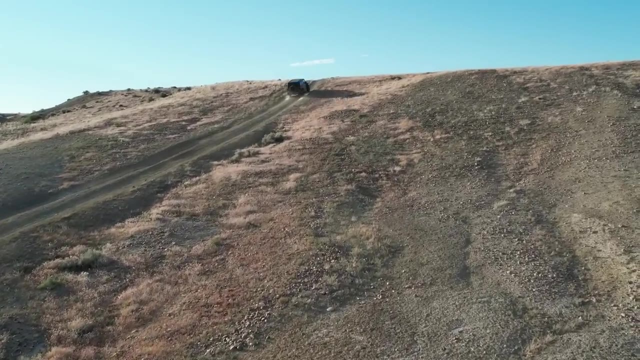 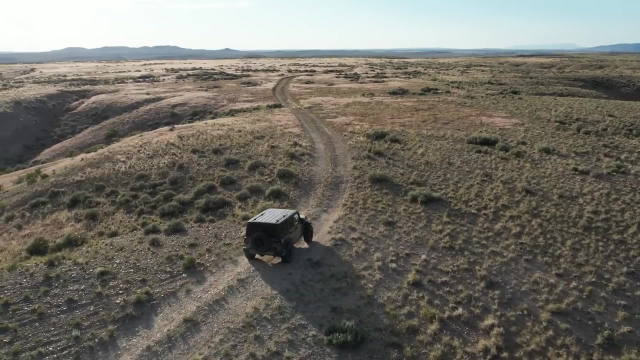 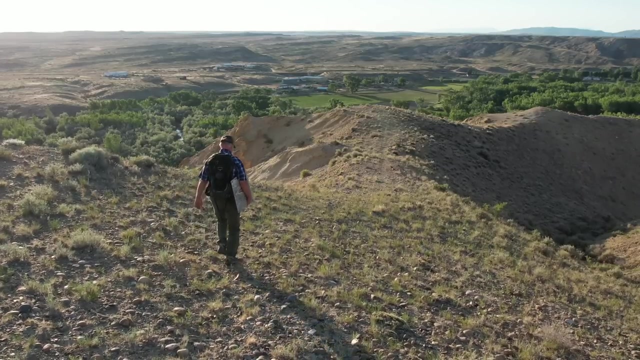 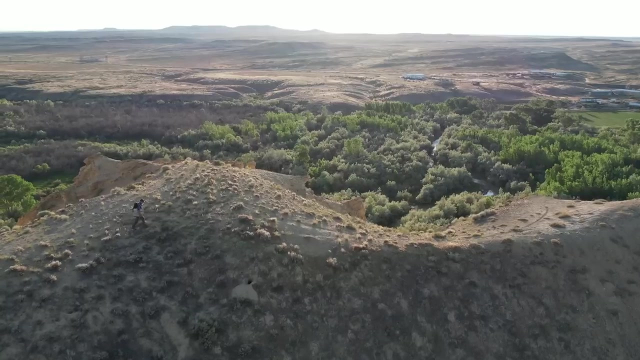 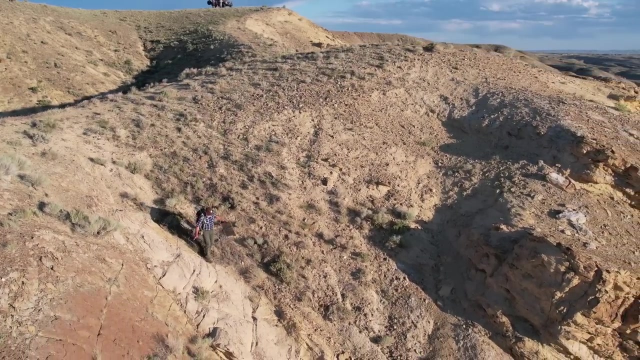 and learn these concepts, Thank you. As I walk down to this rock outcrop, I can't help but ponder the phenomenal history written in the rocks And, as you might guess, this particular location is going to reveal to us some fascinating history of nearby mountains. 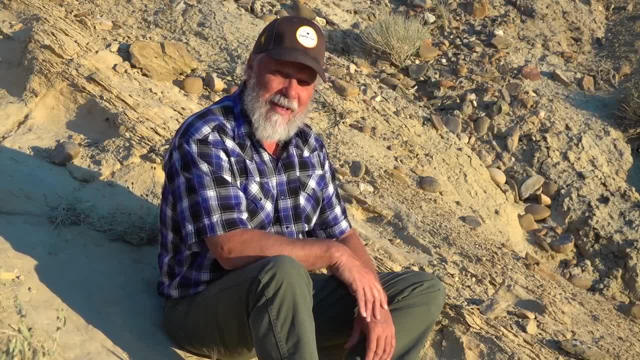 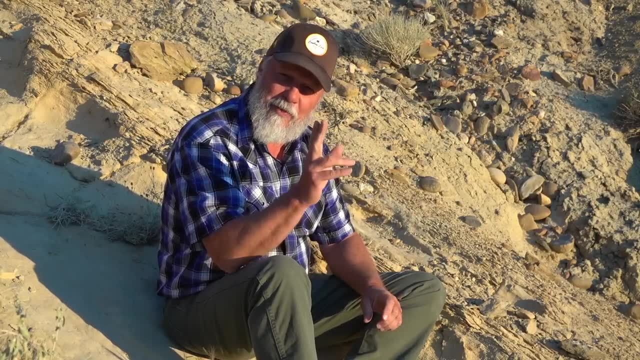 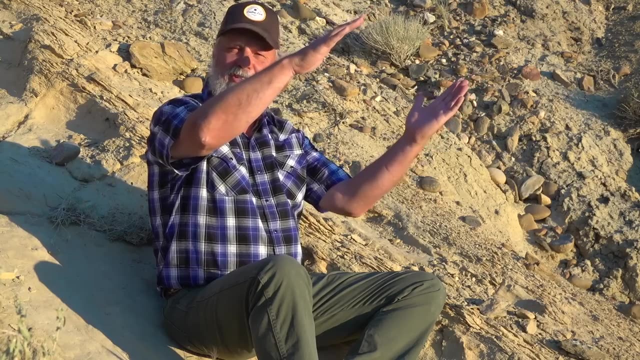 So I've made it here to the Bighorn Basin, to my home near the town of Basin, actually along the Grebel River And this really interesting outcrop, which I hope you'll appreciate at the end of this discussion. I've shown you these beautiful formations that are dipping and that, at one time at least, went up and over the Wind River Mountains. 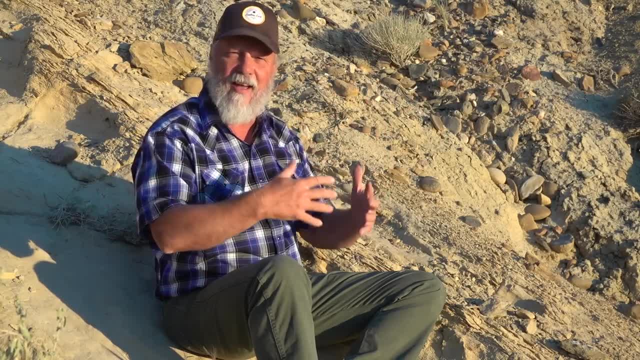 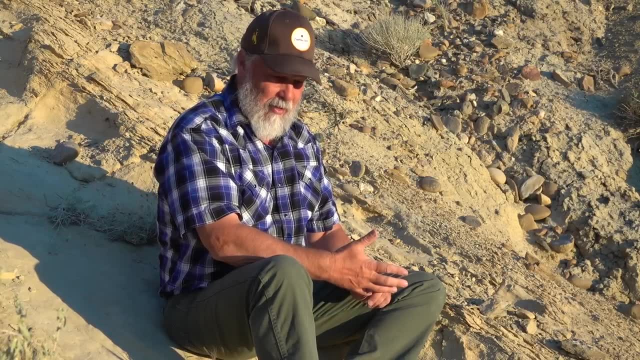 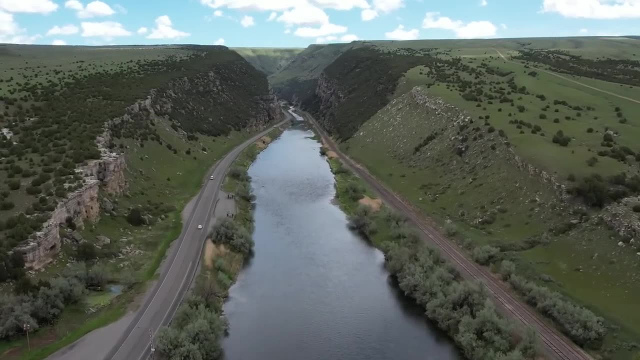 Erosion has stripped them back one layer at a time, right down deep into the mountain right. And if you see some of my other videos, you'll see that some similar views on the Bighorn Mountains, the Owl Creek Mountains and even the Beartooth Uplift near Clark's Canyon. 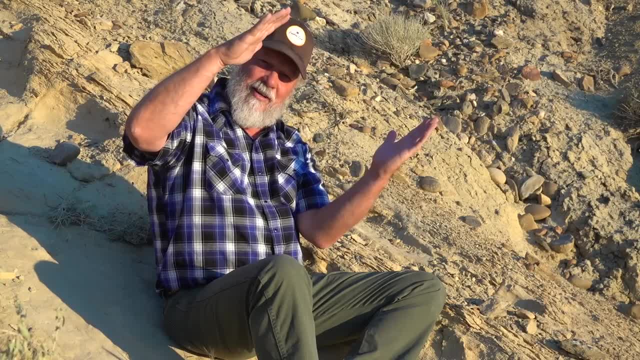 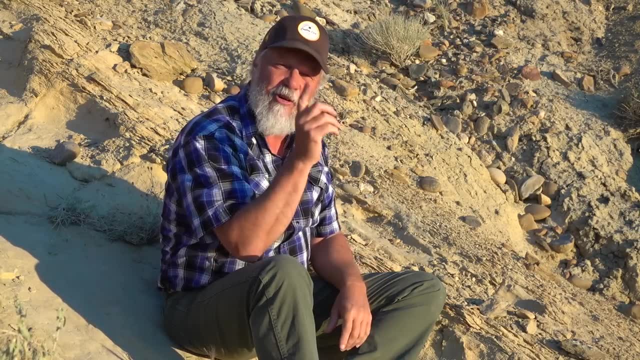 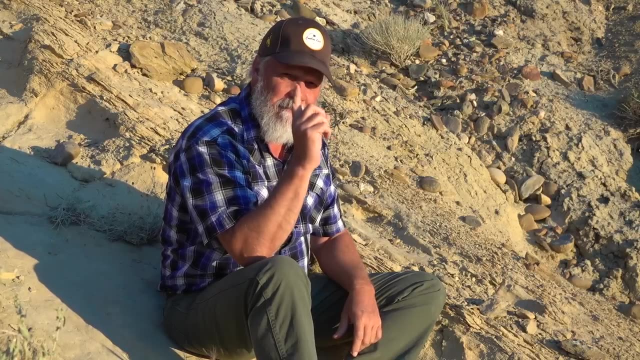 You'll see these formations that are spectacular, Just beautiful thick formations dipping up to the peaks of the mountain. right, It turns out, if we study these formation layers, we can tell an awful lot using one very simple geologic rule, should we say. 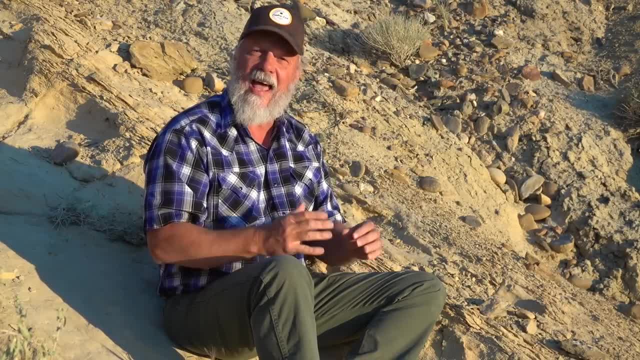 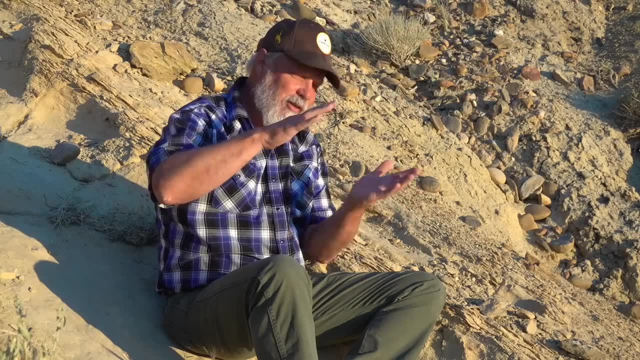 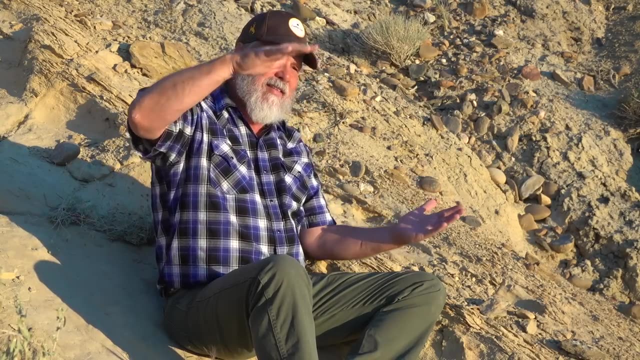 Or geologic principle, And that is- is that originally everything was deposited horizontally and at the larger scale. Yes, small little bed forms and things you know at a small scale can have dip to them, But by the time you get up to you know tens of feet or more, these layers were deposited horizontally. 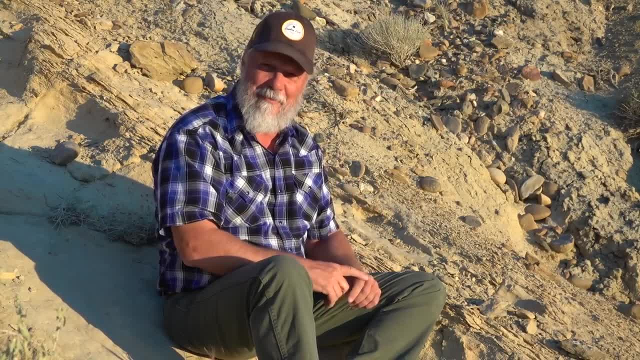 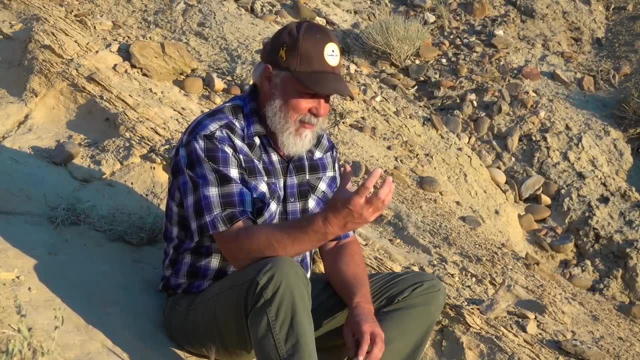 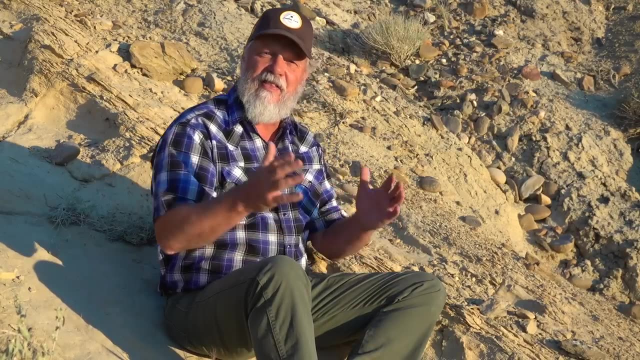 That's a fundamental principle And I've touched on that before, as some of you know. This is what I mean. This is what I really like about geology is that if you understand some basic concepts, you can sort through some really fascinating outcrops in your head and the significance that they have. 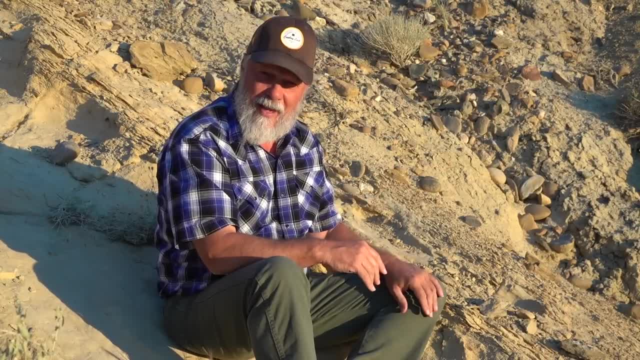 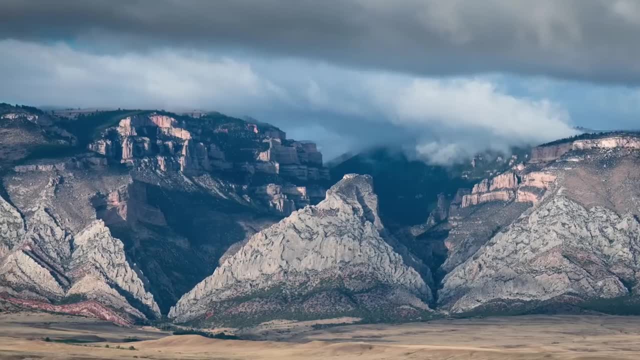 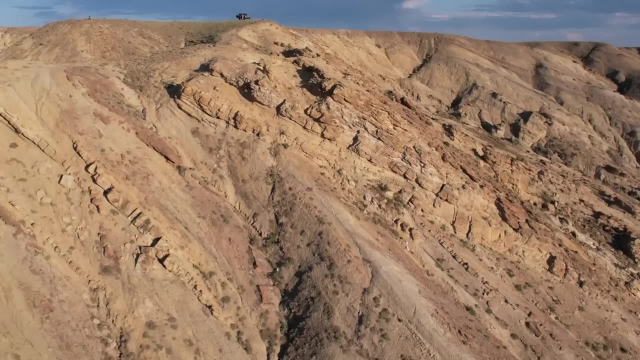 And it turns out, this very outcrop that I'm sitting on tells us when the Bighorn Mountains right behind me, oh, 30 miles behind me when they were uplifted. So let's get into that. This is the key view of the outcrop that I want to talk to. 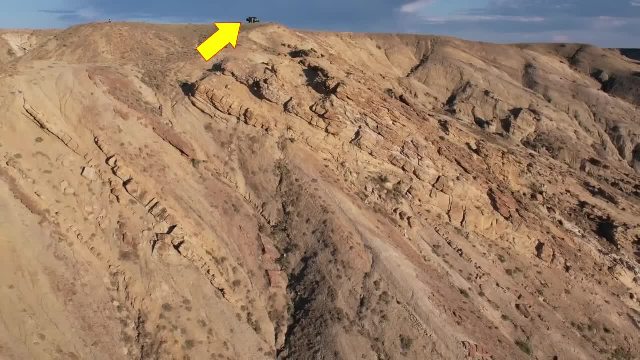 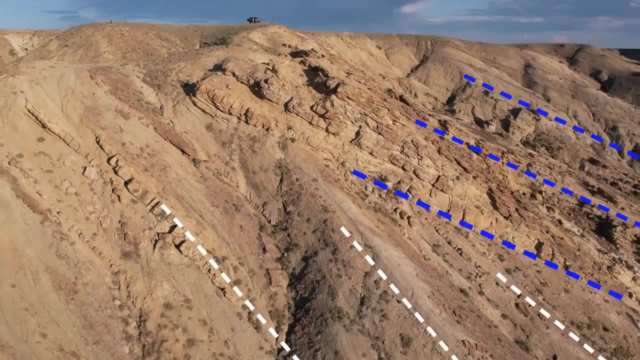 Notice my Jeep up here on the ridge for scale. If you look at this outcrop closely, you will notice that there are layers that slope or dip different amounts. I've drawn lines to help you see what I see. The older layers marked with white dashed lines slope at a steeper angle than the younger layers marked in blue. 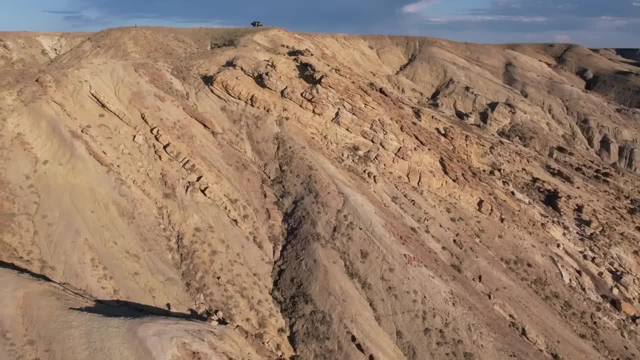 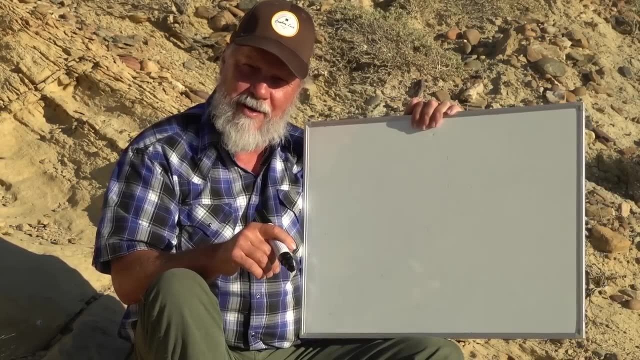 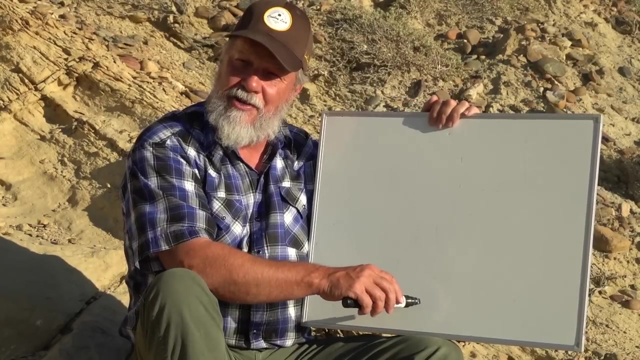 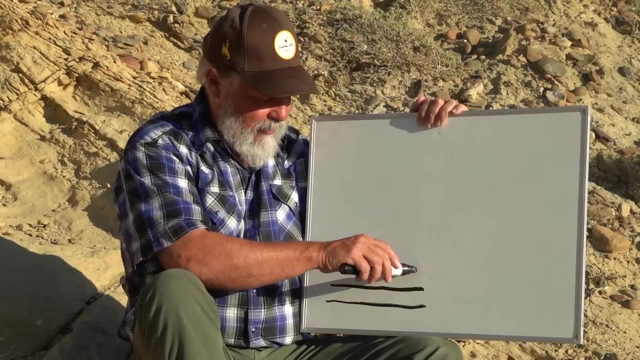 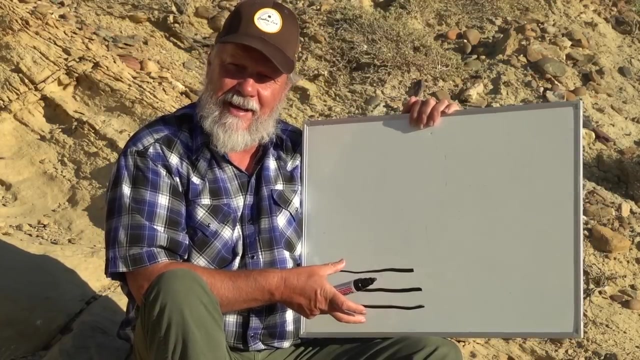 So I'm going to draw a sequence of events here on this whiteboard to help us understand this outcrop that we've observed with the drone. First of all, we deposit layers horizontally right, Layer upon layer upon layer. Okay, And in fact we deposited about 11,000 feet of rock horizontally like this before the Bighorn Mountains started to uplift. 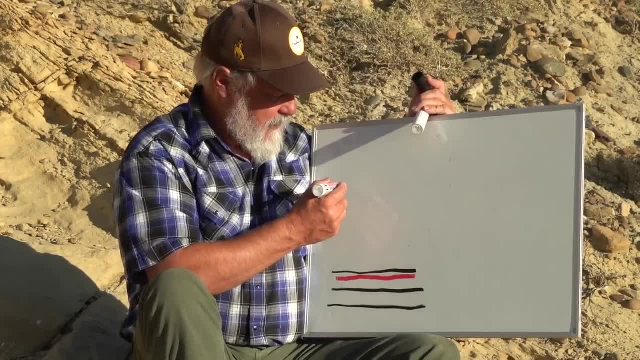 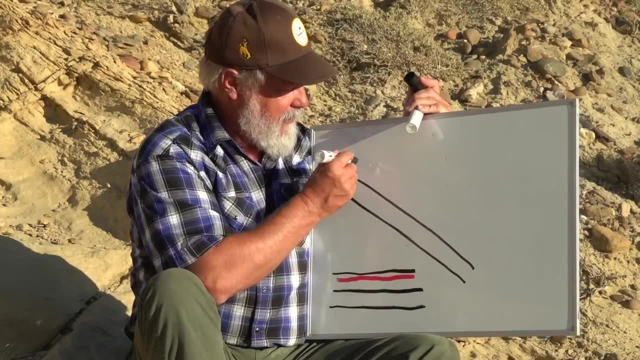 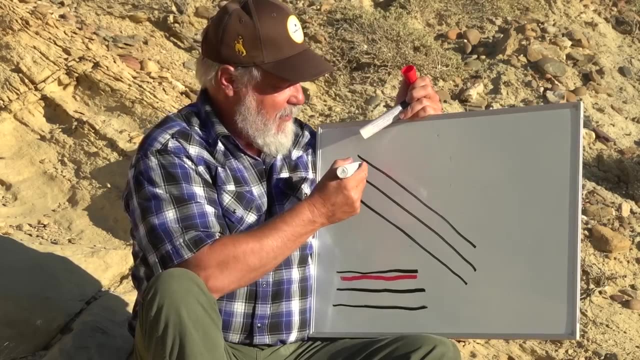 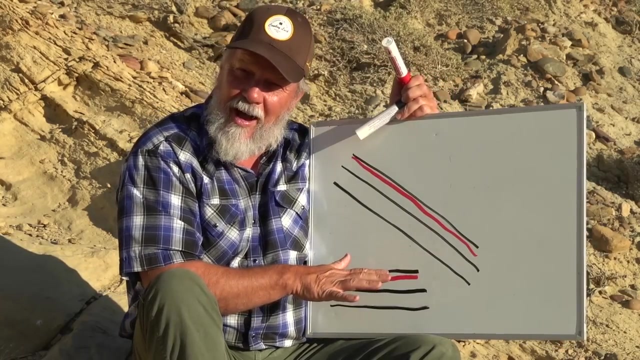 And now the uplift starts to occur And I'll tip these layers like so One, you know, just like that, And I'll put my little red bed in there for reference, like this. So we've taken these horizontal rocks, these big formations, like I say, 11,000 feet. 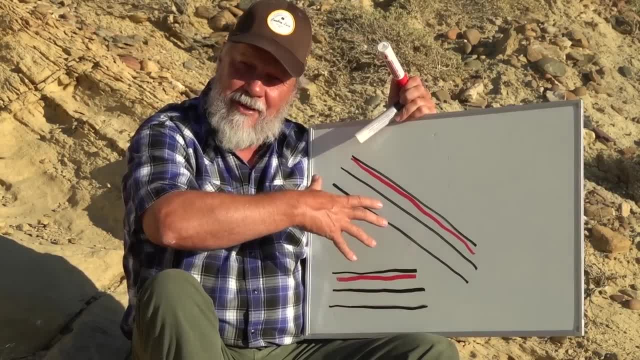 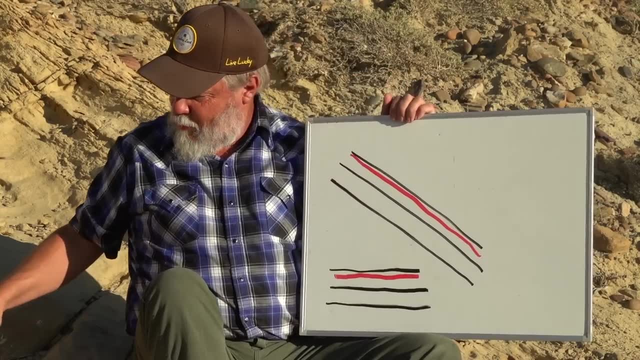 And we've tipped them up as the mountains were uplifted. It's all pretty simple, right? And what happens when we start tilting rocks and uplifting them? Well, we start to erode because we bring them up, So erosion comes in. 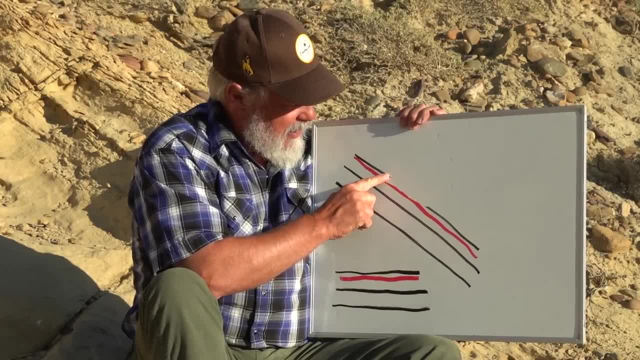 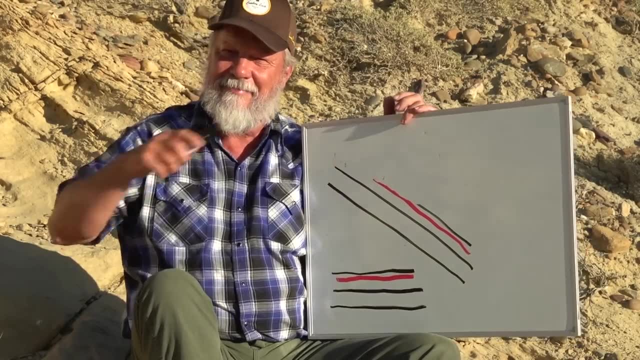 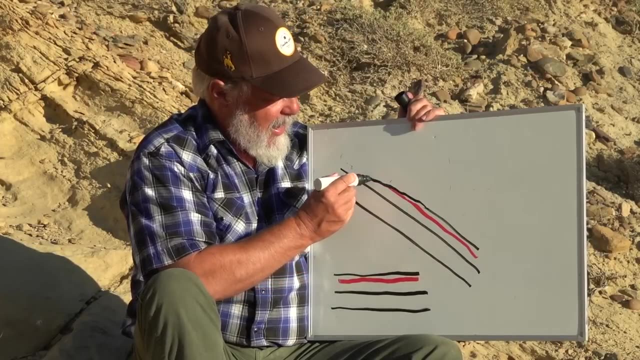 Huh, okay, And it starts to erode, And maybe cutting out this like that, Let me draw an erosion surface there- So it erodes out. That's why I drew this little red bed here. okay, It erodes that out and kind of cuts it off, a little like that. 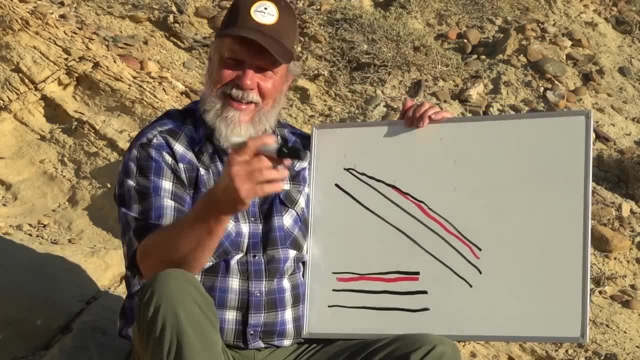 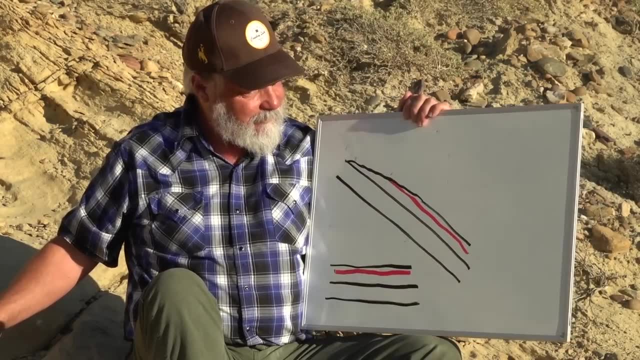 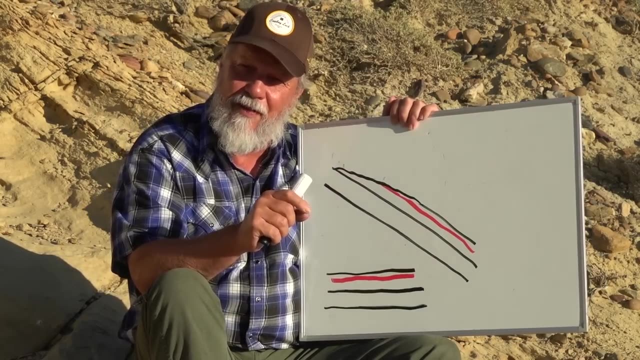 As it's being uplifted, these rock layers. See, this is really pretty basic, isn't it? But now the important thing, As, yes, these rocks have tipped up, But deposition continues to occur on the flanks, On the sides of these beds. 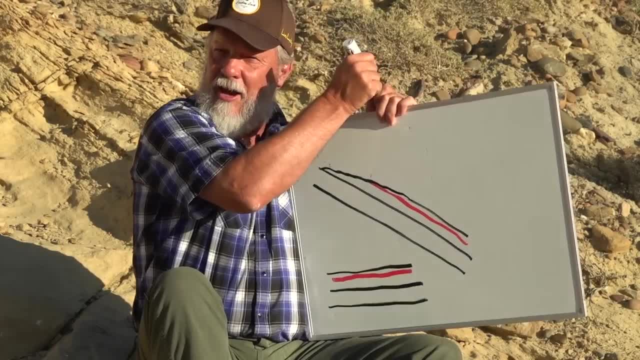 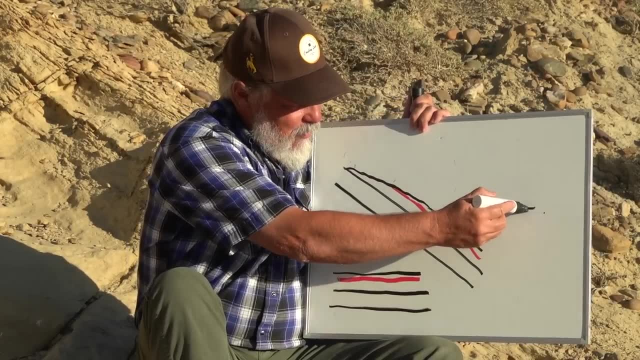 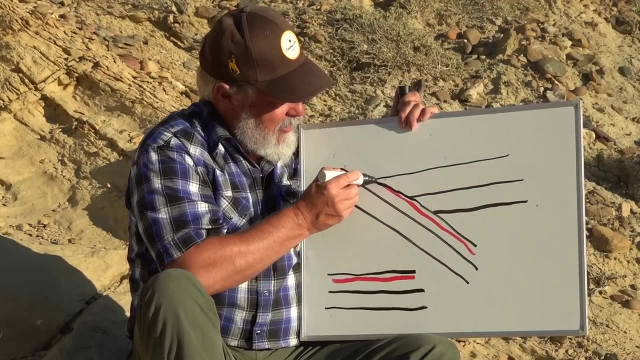 These big formations. And it's coming in horizontally, isn't it? We use the same principles, right, And I'll try to draw horizontally. here We come across And it just keeps being deposited like this. Okay, Just keeps filling in. 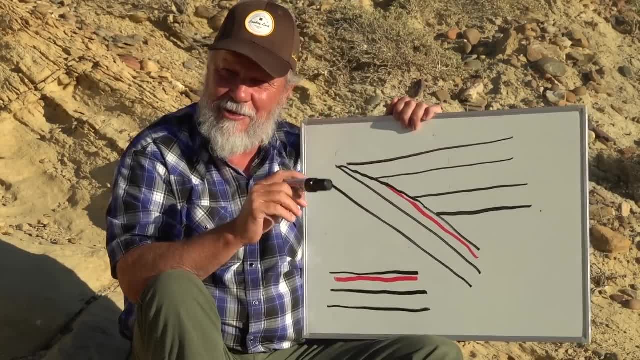 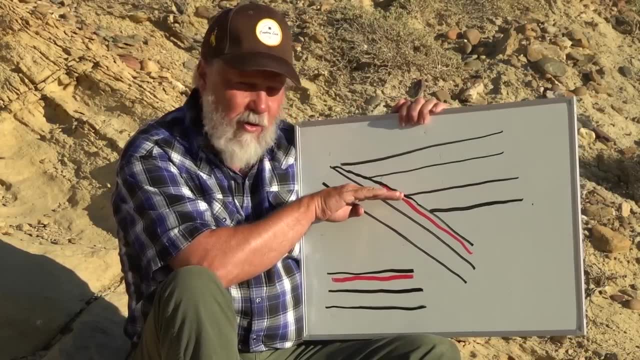 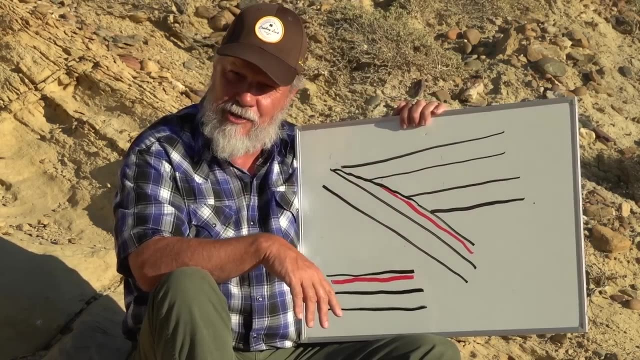 Okay, Now we're starting to get to some critical information, And that critical information is that we've cut off some of this, We've eroded it off And we've deposited on the sides like this. In my world we call it an on-lap surface. 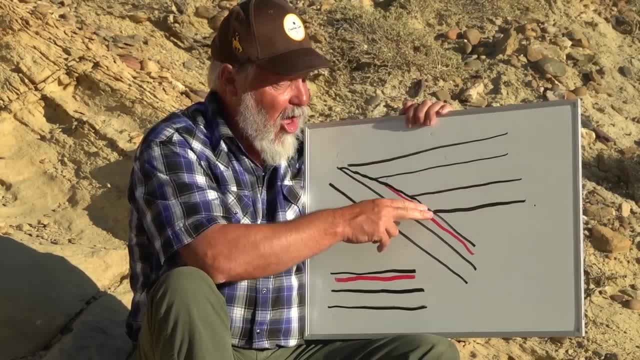 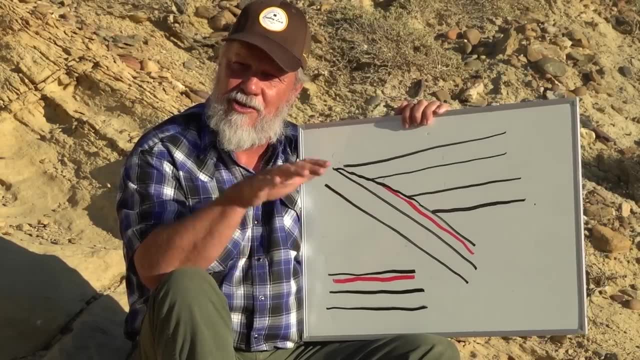 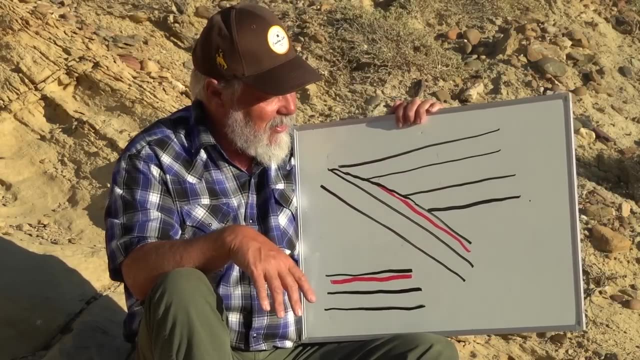 Because these sediments that are being deposited on-lap, this dipping surface- And I've had the great fortune of seeing this in seismic data, Which is underground geology From seismic All over the world. It's beautiful And I've had the great opportunity of unraveling many geologic stories in the rock record. 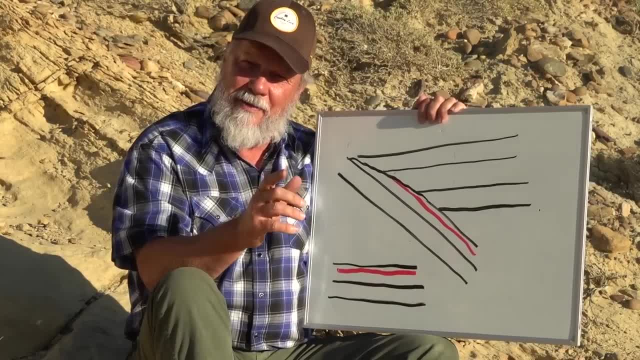 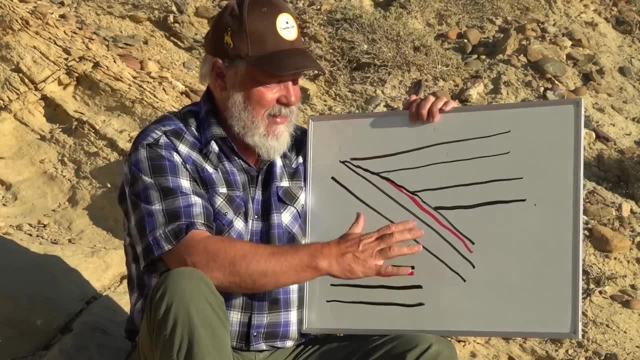 Using some of these techniques. Okay, So now we're set up, We're getting close to what this outcrop is showing us. Of course, the mountain didn't just uplift to here and stop. It continued to go, It continued to uplift. 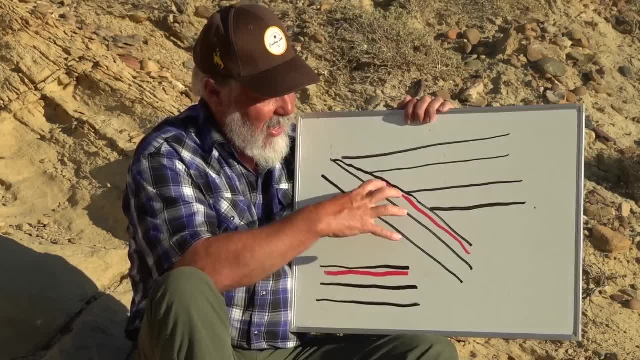 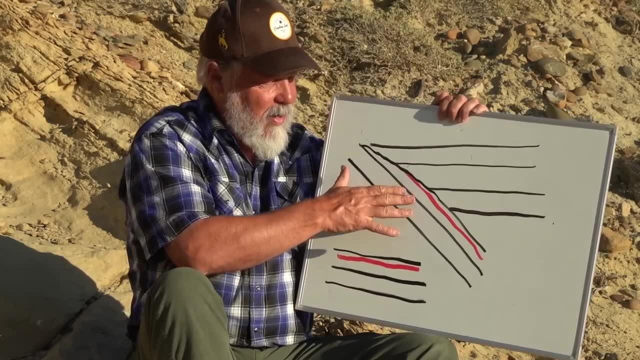 And what I'm going to do is just rotate this whiteboard to show that. So here we are: at this time period, We've eroded, We've put in some sediment And the uplift continues to go And tip this rock even more. 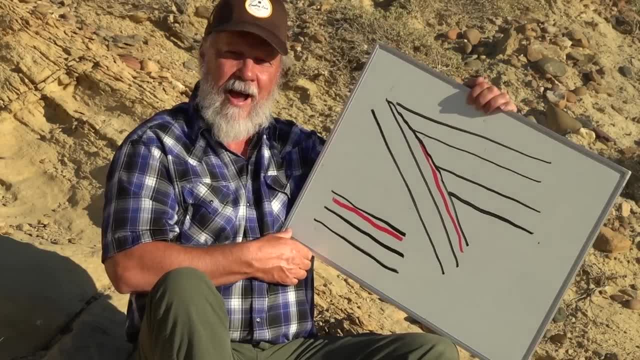 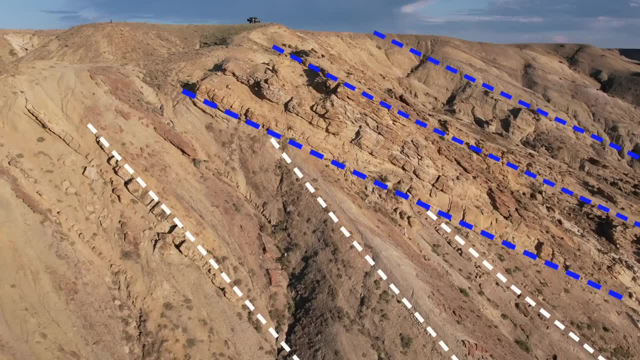 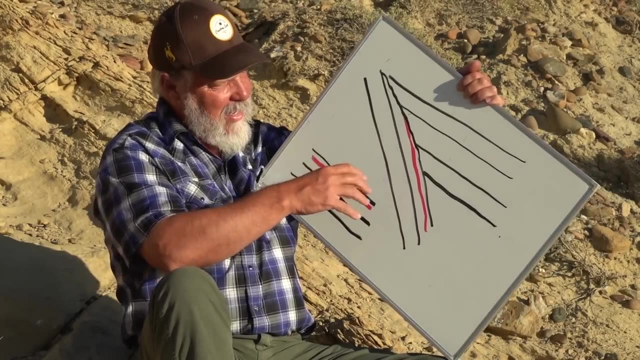 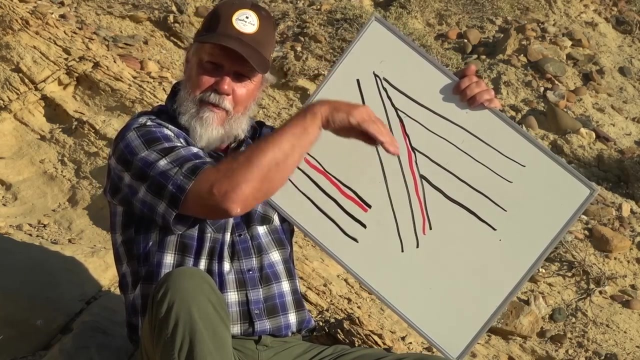 More And more And more And more. Finally it stops And this outcrop is recorded. obviously, after it stopped It's recorded. So let me do this. Oh, this is a bit tricky. here Now we have both. all these layers are dipping or sloping this way up towards the Bighorn Mountains. 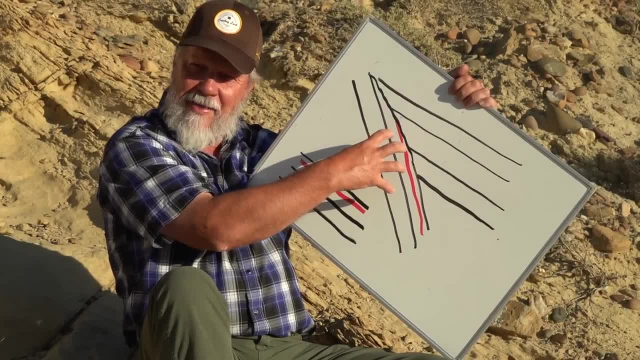 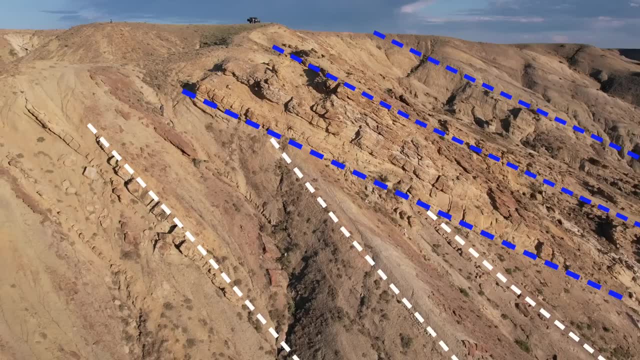 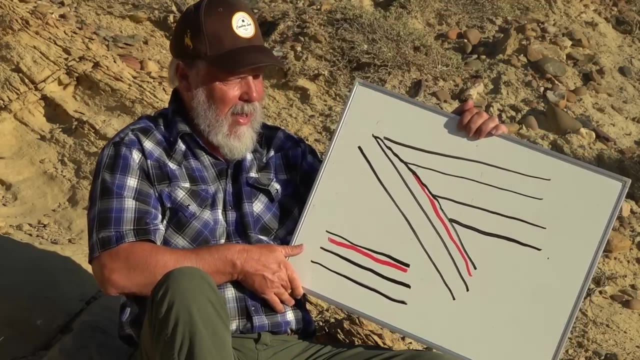 But some, these old layers, this 11,000 feet that I've mentioned, they're tipping more than these And that's why, Because they started more tipped, They started here after the first pulse And then the mountain building continued to here. 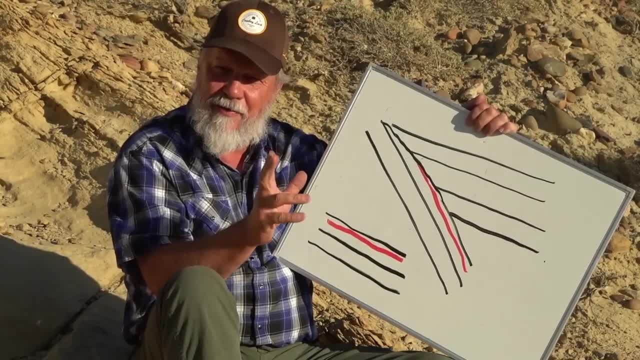 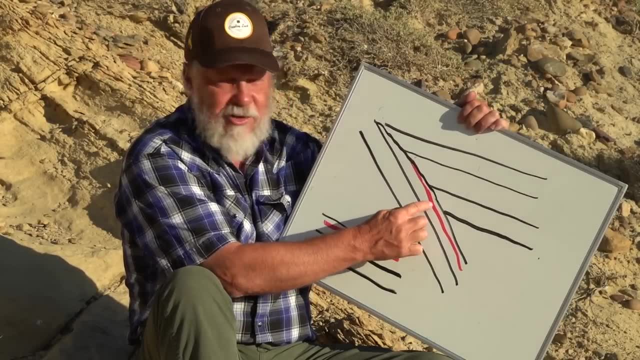 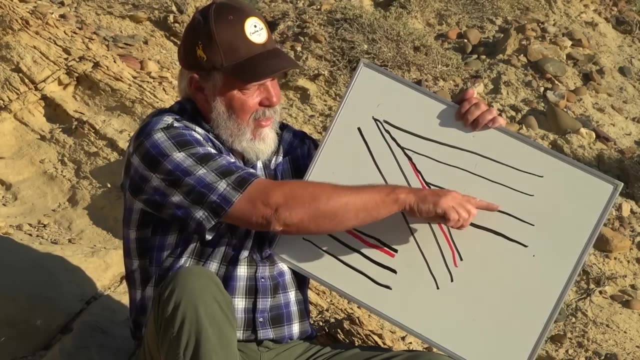 And now we have the critical observations that we see in the drone video, And that is, we see some layers here that get cut, like this red layer. That's why I have that in here. It's cut off And we have this surface right here that everything comes to. 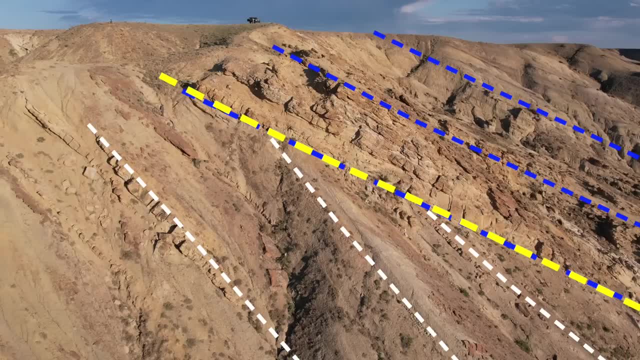 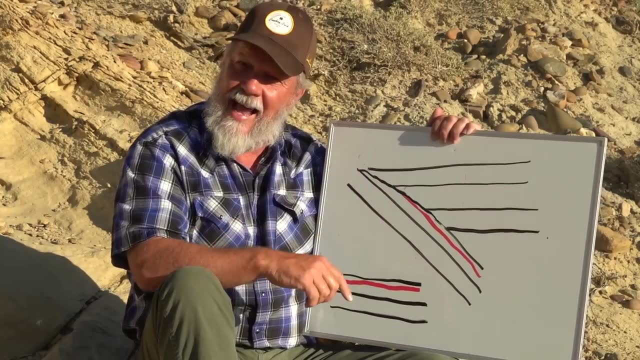 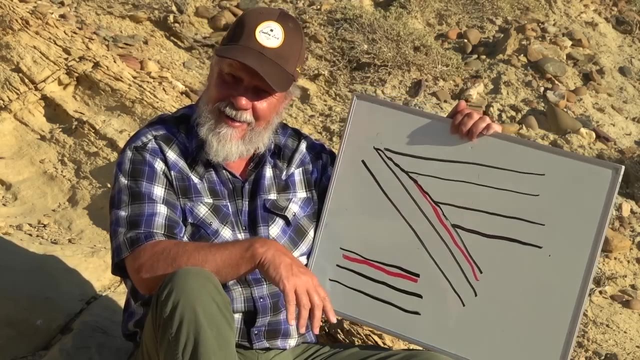 That is the unconformity, And this is called an angular unconformity because the rocks are at different angles. coming into that contact, This unconformity, And also erosional. It's been somewhat eroded here, So I pull this up here, my stratigraphic column. 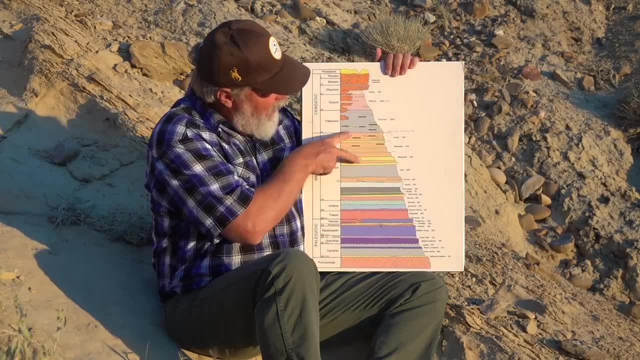 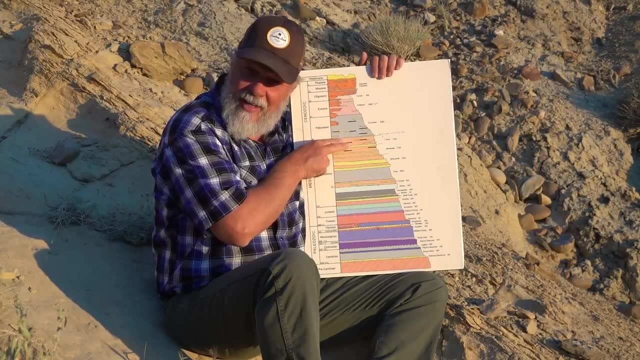 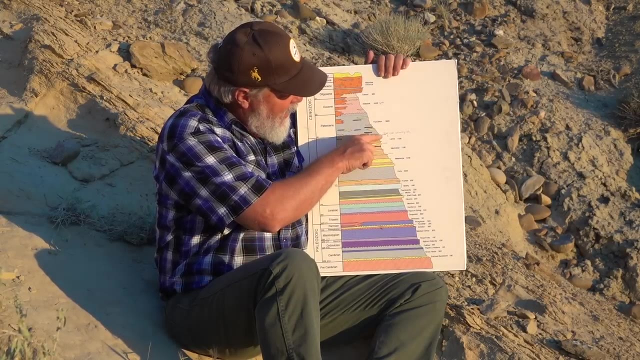 And this formation here is called, yeah, the lance formation, the upper part of it. Okay, It's Cretaceous age, Okay, It's just older than 65 million years old, And that contact, right here, is where this is. 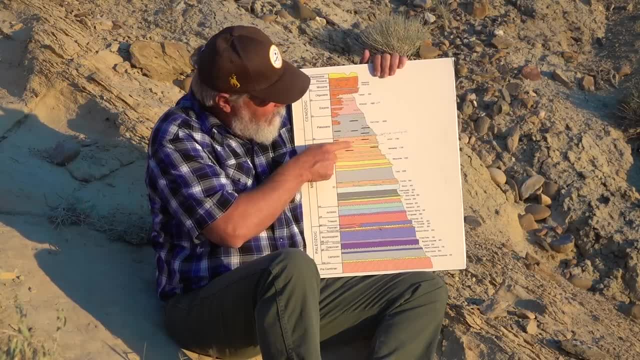 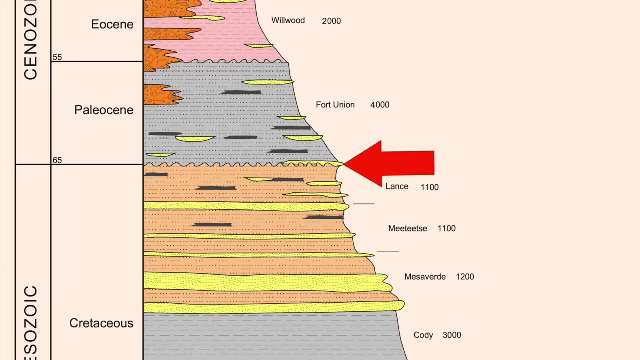 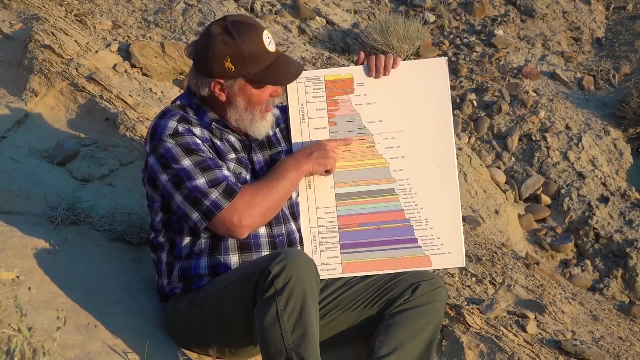 Right. here is where this unconformity is, Right at the top of this orange lance formation, And above that are these gray layers that I show in this stratigraphic column that I made. It's called the Fort Union formation. So all these layers, this is the neat thing. 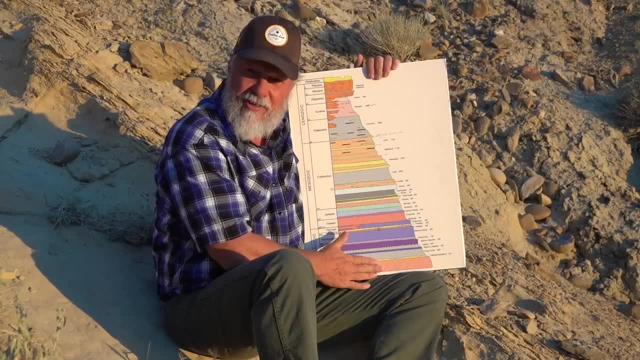 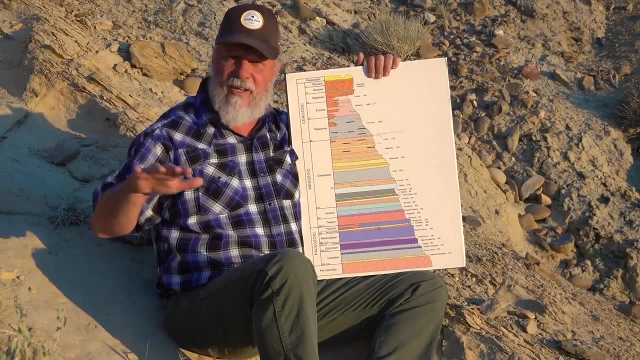 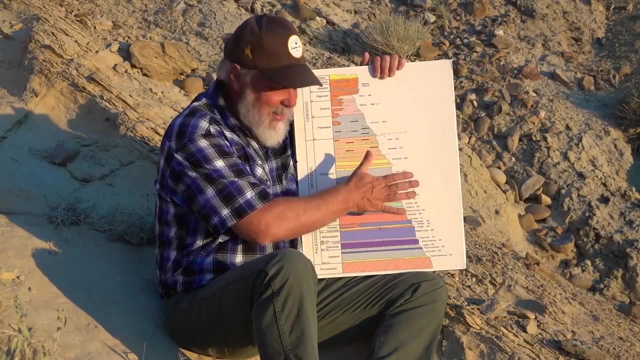 All these layers from here down existed prior to the uplift of the Bighorn Mountains. They extended over a huge region all around here and were horizontal. Okay, They hadn't been touched, so to speak. They had been deposited horizontally and not tilted at all. 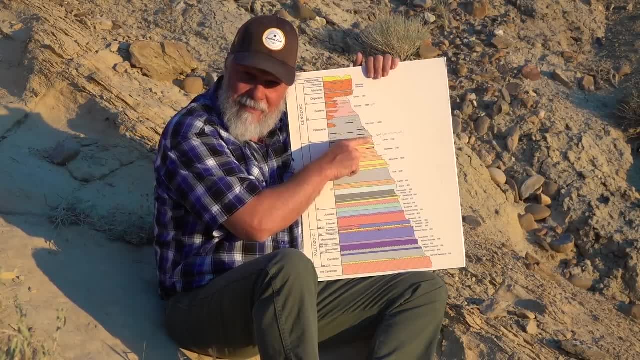 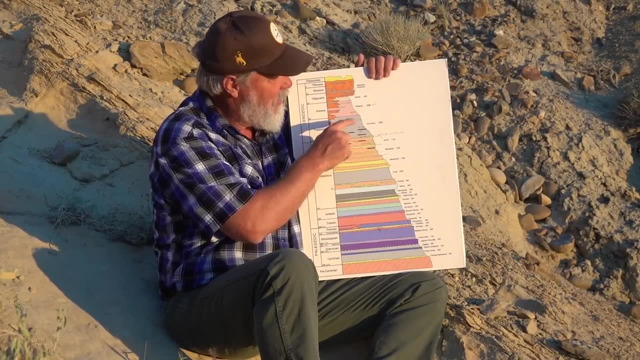 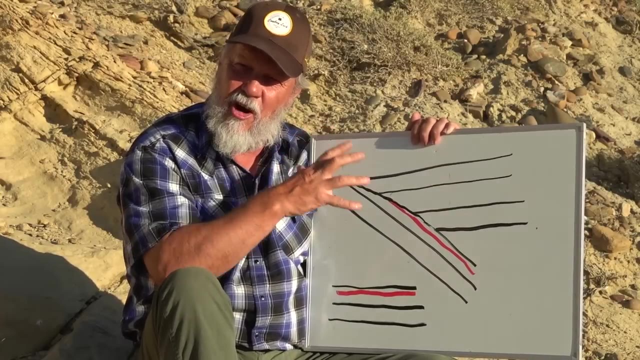 And then, right at 65 million years ago, they started uplifting And that is that unconformity between the lance formation and the Fort Union. So I hope that helps you understand this outcrop And the history, the early history of the Bighorn Mountains. 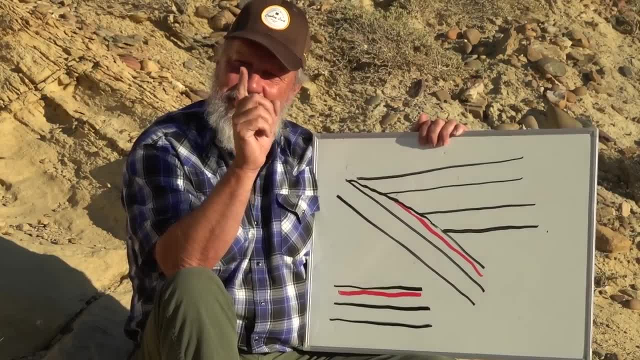 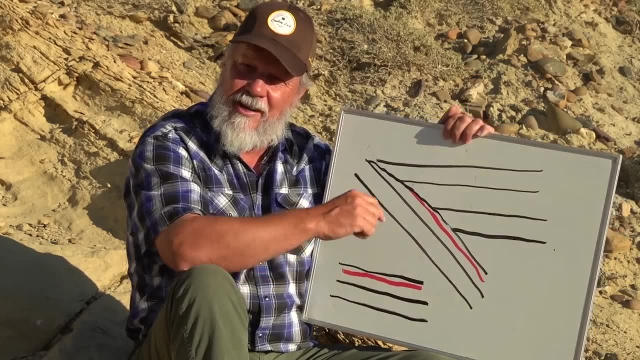 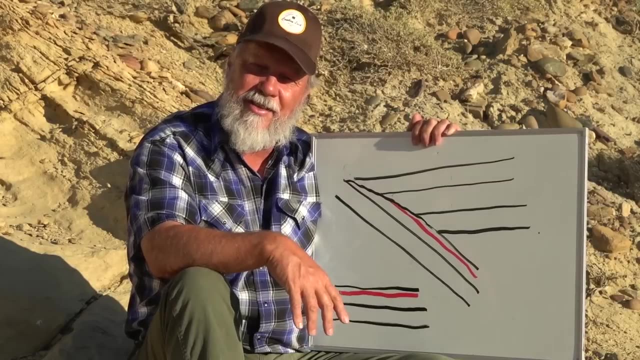 One other fascinating point I want to make. It turns out that right during this time of this uplift here and erosion and the formation of this unconformity, You know what happened? Chicxulub, that great asteroid that came and impacted the earth at the Yucatan Peninsula, occurred. 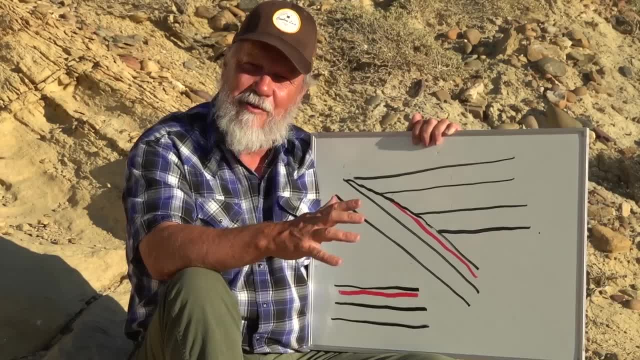 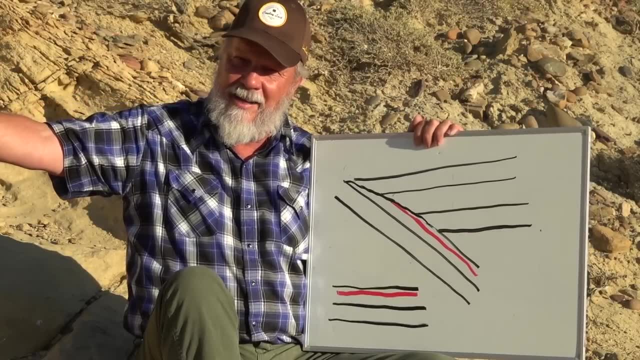 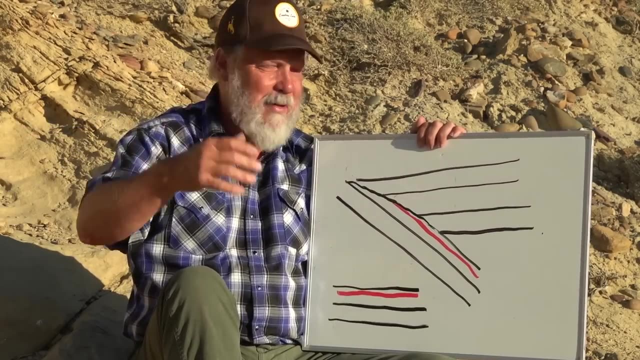 And wiped out the dinosaurs. So what that really means is all the rock that I'm sitting on and back to my right here is the older rock. Dinosaurs were happy, At least you know, for a period here, back here, Starting in, say, the Jurassic and coming up. 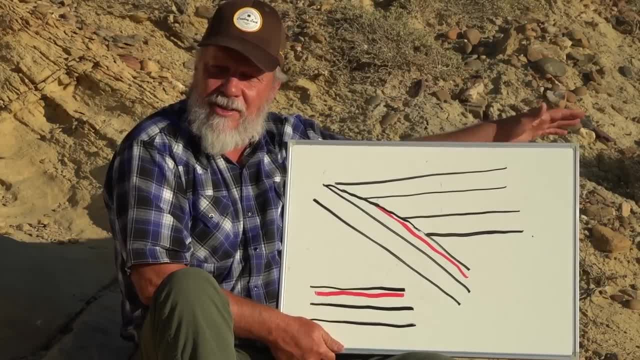 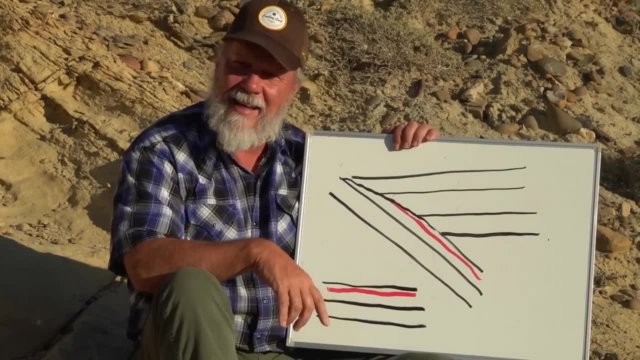 And on this side up over here that we've seen on the video. I can't point to it quite directly here. Up there, just right over here, a few feet from there up, dinosaurs are gone. It's an amazing contact. 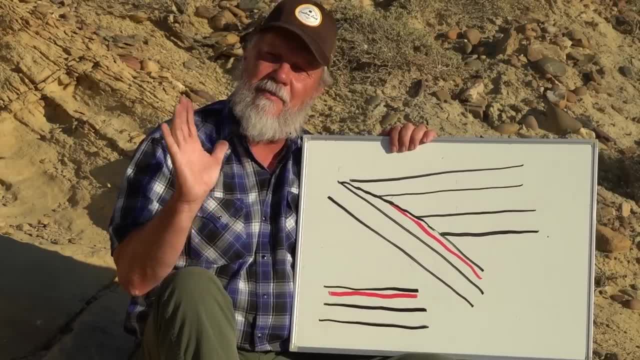 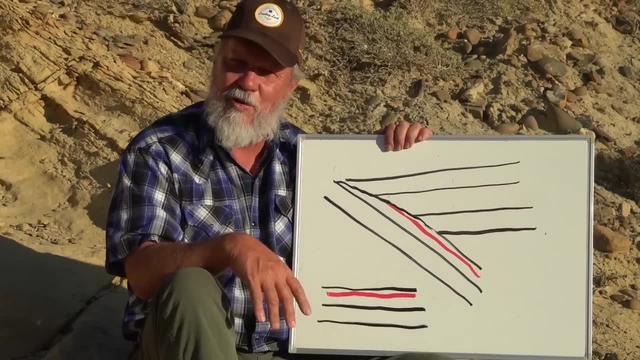 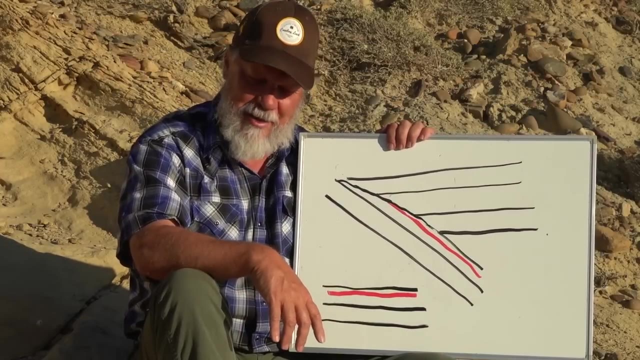 One point I want to make is that the formation of the Bighorn Mountains wasn't caused by the impact crater Or didn't cause the extinction of the dinosaurs. It just so happened. it was occurring right when that meteor hit the earth. But using radiometric dating, which I have mentioned, I don't want to get into. 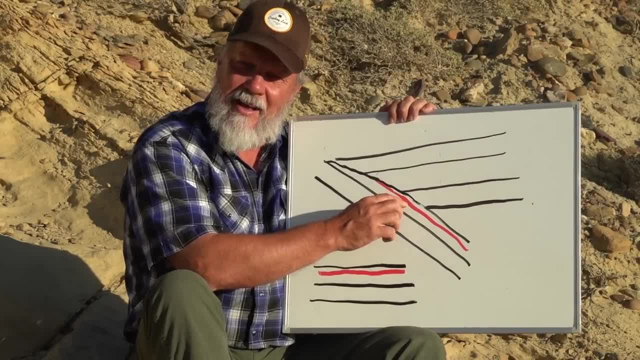 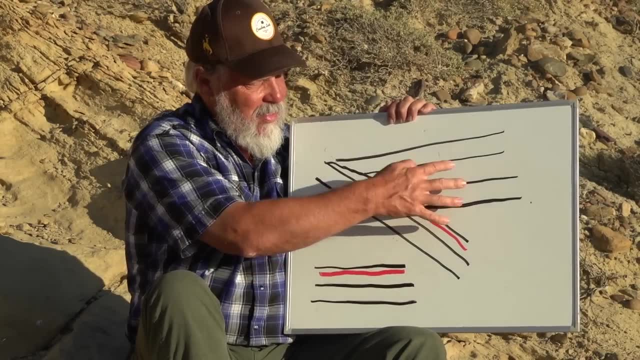 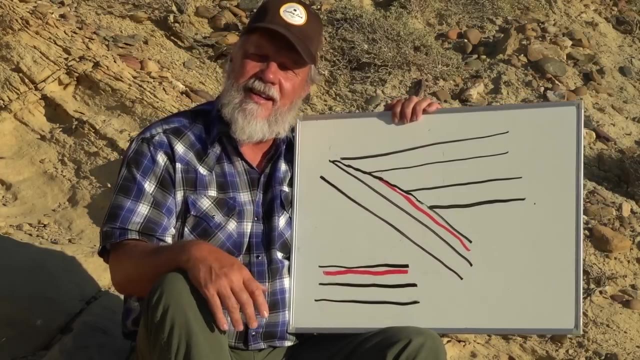 We know that the age of this formation, When it was finishing up being deposited, was about 65 million years ago, And we know when, so that tells us when the uplift started to occur, Even if we discard radiometric dating and just not worry about it. 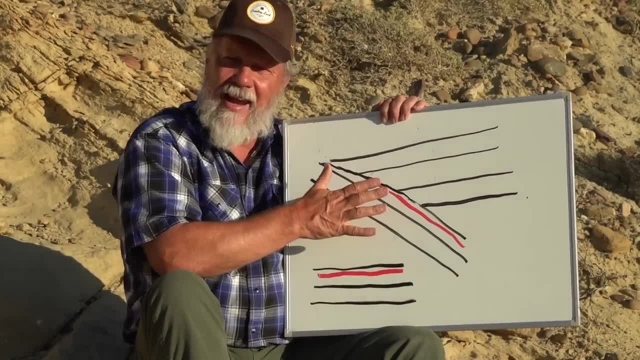 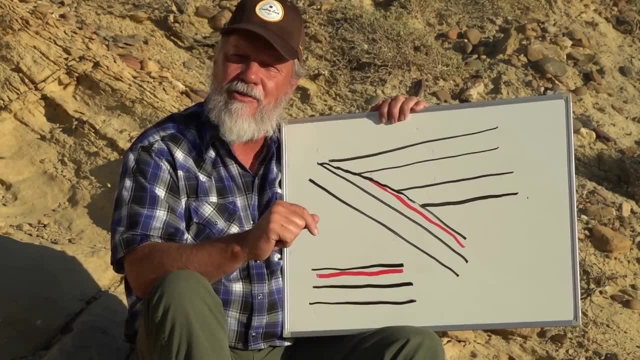 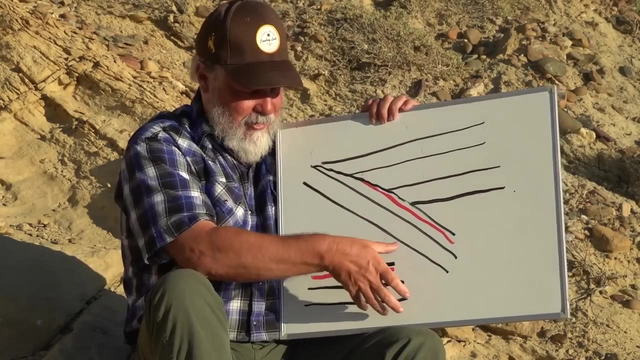 We can tell so much And we can figure out relative to deposition and relative to new layers coming in When the Bighorn Mountains came- And this is what this has done right- It's shown us that these layers were deposited first. 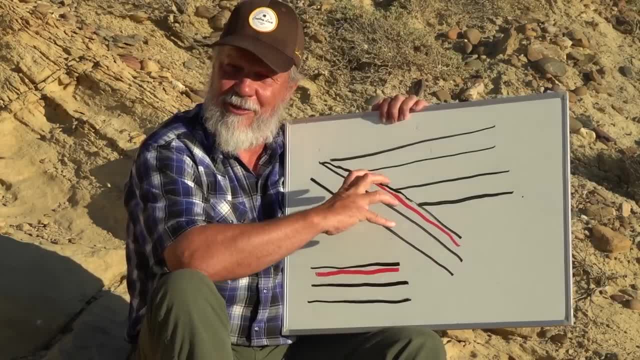 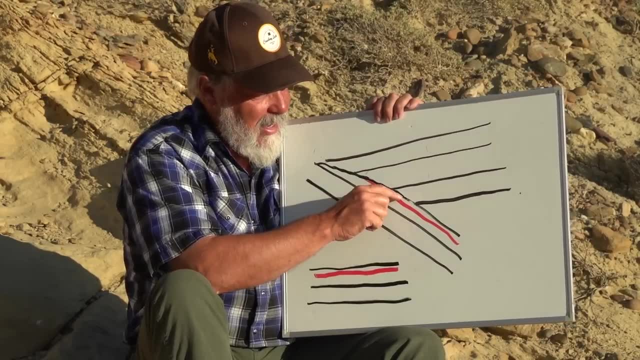 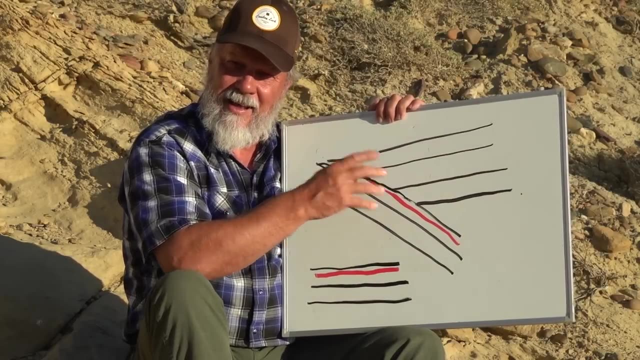 All these old layers that were then tilted And then, relative to the age of those formations, Whatever they happened to be, Right here at this age, Right after this layer was deposited and the new layers came in. That's when the uplift occurred. 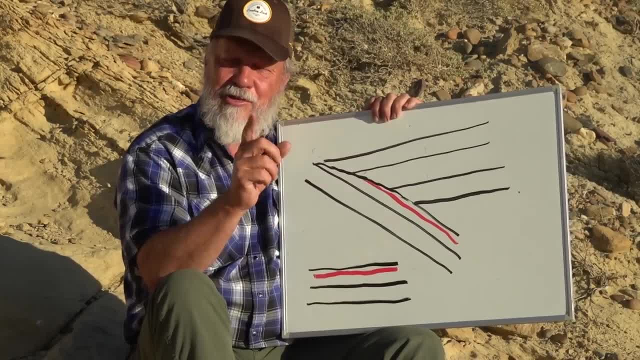 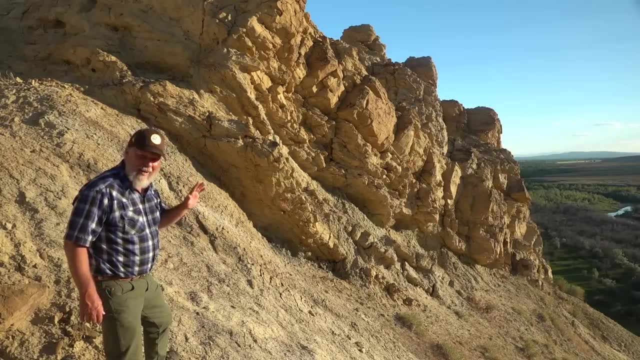 And we can worry about the precise absoluteness, But we don't want to re-date later, can we? This is quite steep, But I wanted to walk over. I love to put my hand on these contacts, On these contacts, These unconformities and things. 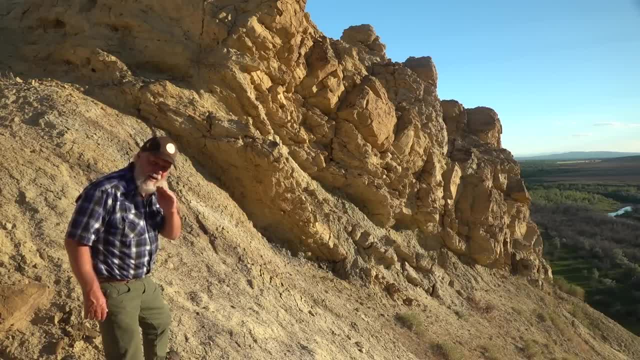 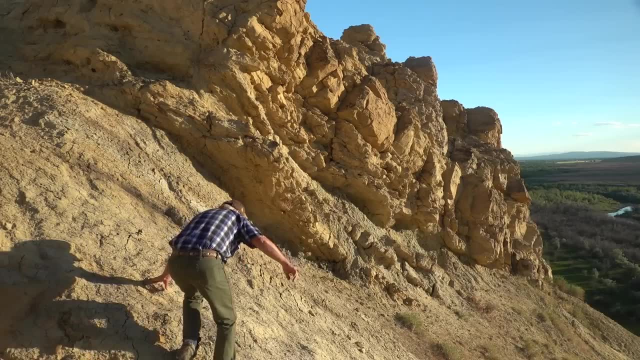 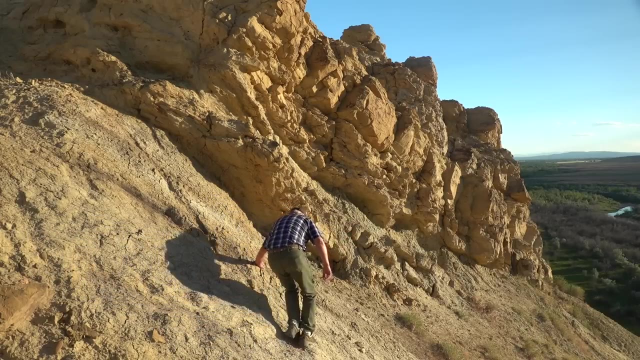 These geologic contacts. I'm going to try to scramble over here and put my hand right on that unconformity Where we have so much history. That's about as steep a slope as I want. Fortunately, there's nothing dangerous here. 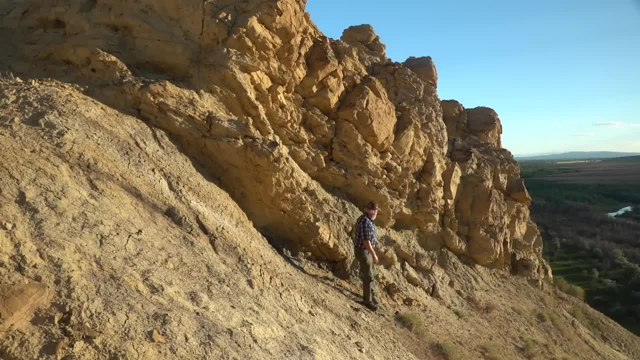 Don't get too worried about it, But I'm getting close to the contact. So right here, Right at the base of this sandstone that we see in the drone video, Right here, These are where the new sediments, The new layers that came in at the time as the mountain was starting the uplift. 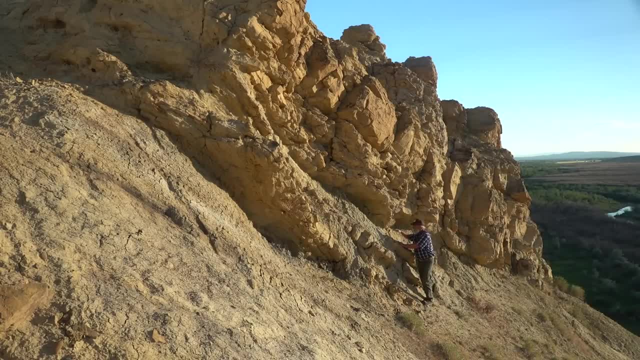 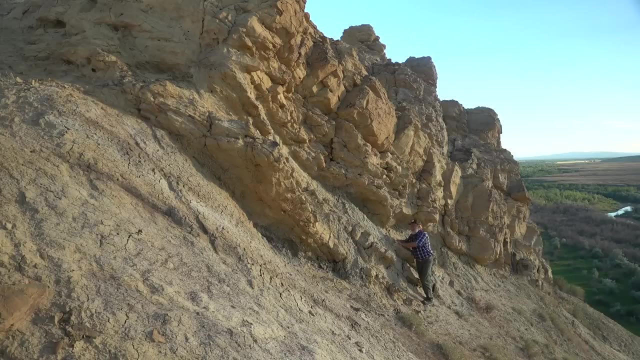 Had started pretty good, Came in onto this unconformity here And then, as I mentioned, As the mountain continued to uplift, These rocks all continued to tip even more, And so you have this angular unconformity Right here And right during this period is when Chicxulub hit. 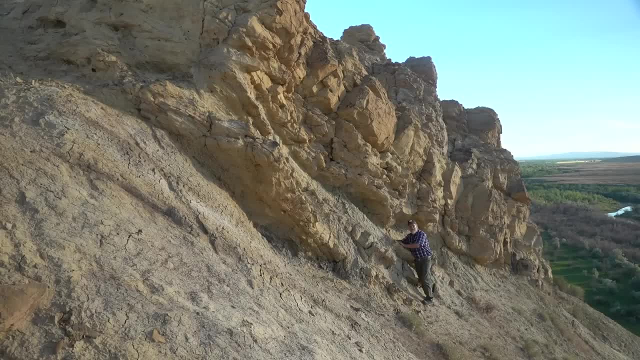 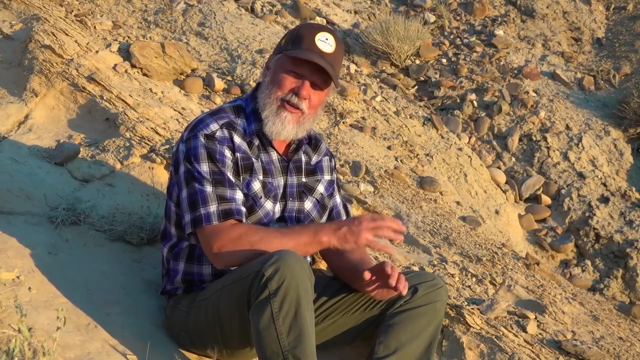 That I mentioned And when the dinosaurs all disappeared 65 million years ago Right there in that vicinity- Amazing history, And it's really cool to put your hand on that contact. Well, Let's go on to this, To the next outcrop. 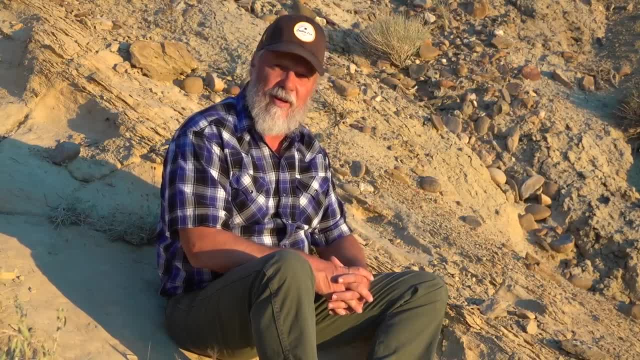 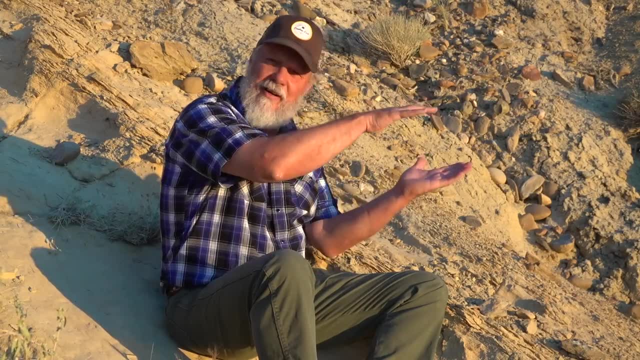 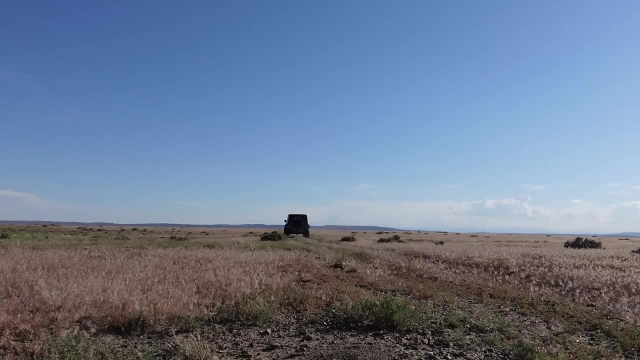 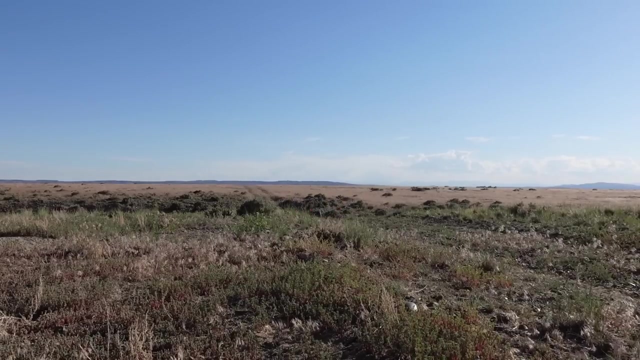 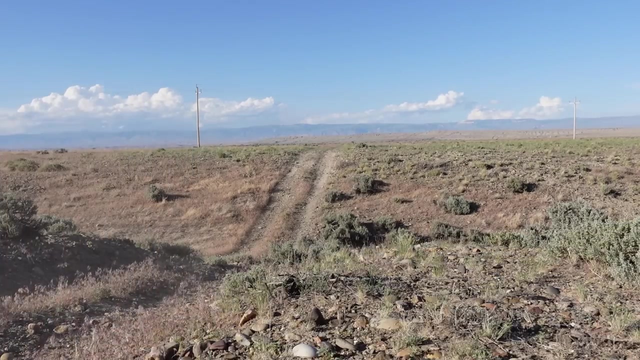 And using these same principles that we just applied here, We're going to see how the Bighorn Mountains Stopped being uplifted And how it was recorded In the history of the formations. Well, I've made it, finally, to the last stop. 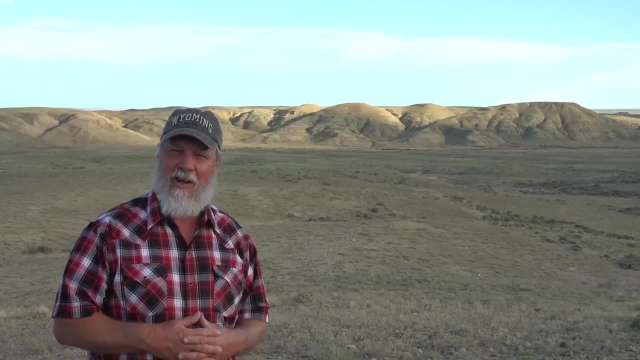 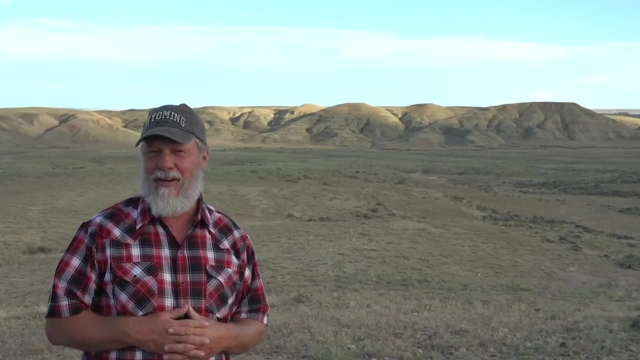 That we're going to do in this video- And this is my favorite outcrop, actually, Primarily because I found it very recently And it's so neat How it records The history of the Bighorn Mountains When they stopped uplifting. 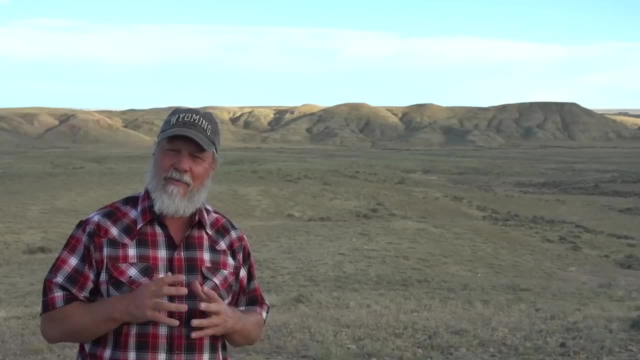 And so it's the end of the Laramite Orogeny- More or less At least in this area- Which occurred about 50 million years ago, When the Bighorn Mountains stopped uplifting, And so it's the end of the Laramite Orogeny. 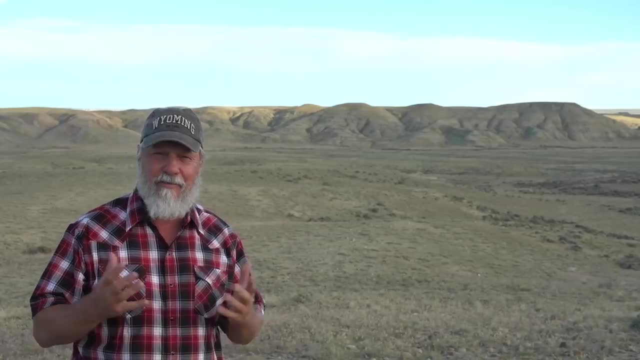 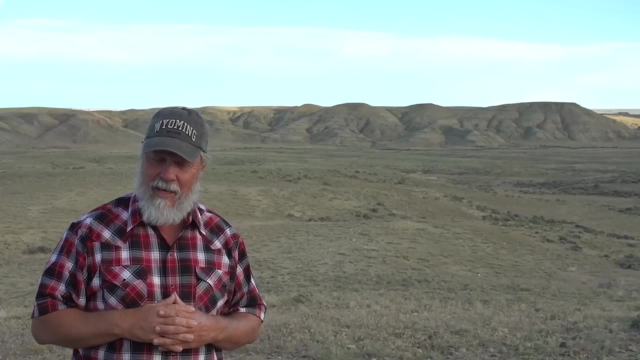 More or less, at least in this area, Which occurred about 50 million years ago, When things shut down. So it started, as we saw, in the last outcrop, If you'll remember, At 65 million years ago And kept going for some 15 million years or so. 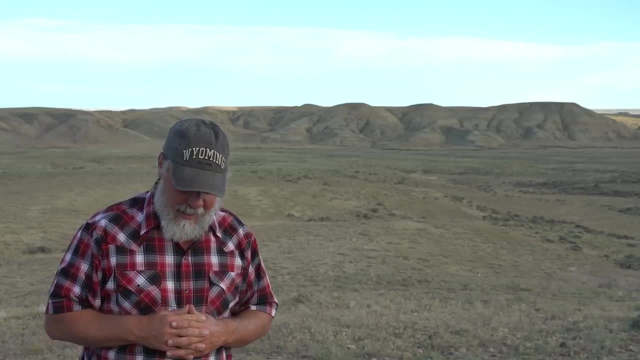 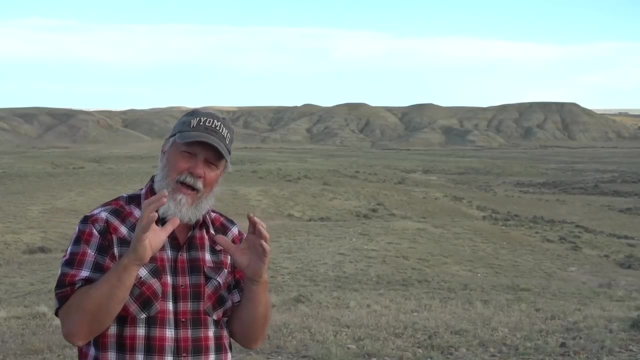 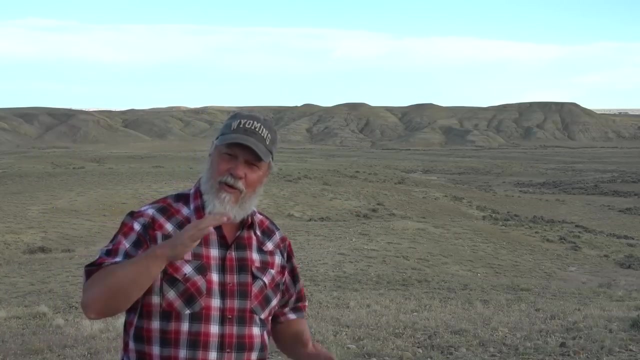 And then shut down And it was recorded in the rock layers. So this is really neat, Because I want you to think about What you might see over there On that ridge With the Bighorn Mountains, The principles that I've showed you, 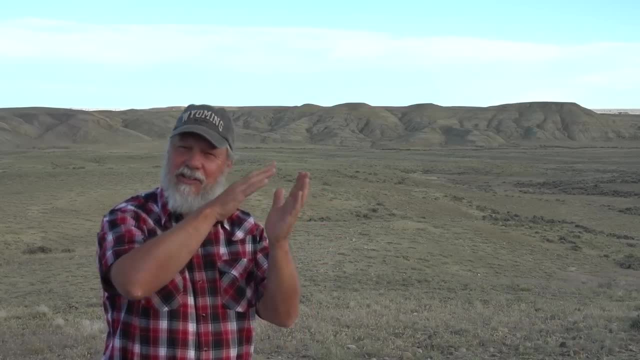 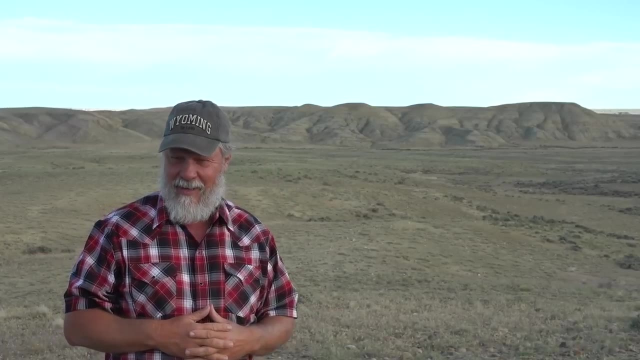 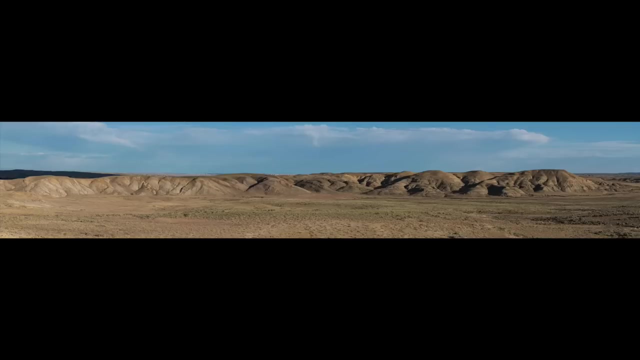 About original horizontality And the deposition, And how the rocks get tilted And then deposition continues, Etc. And what might you see over there As the mountain shuts down? You might ponder that a minute, So let me show you some details. 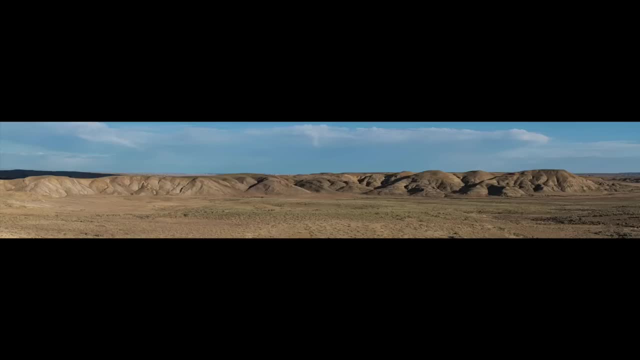 So here we see the full length Of the ridge or hill That we want to look closely at And look for some details. We'll start by zooming in On the yellow square here area And then panning the camera Clear over to the right side of this hill. 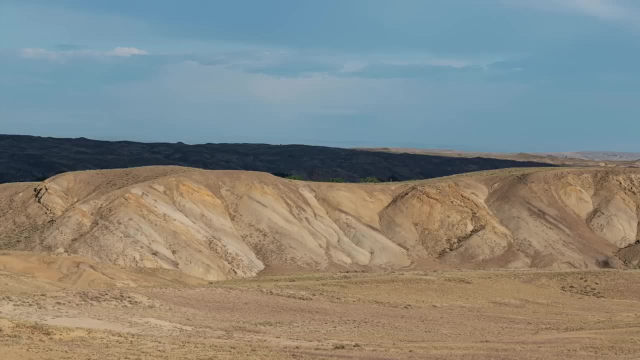 Okay, Let's stop here and take a look. Well, we see some familiar things, Don't we? We see some nice dipping strata Or layers of rock in here. They have been eroded down back. Remember they at one time? 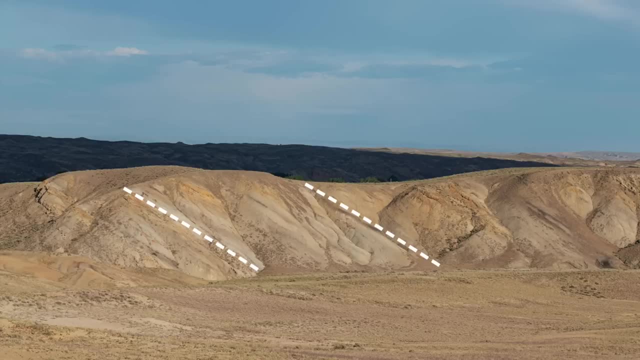 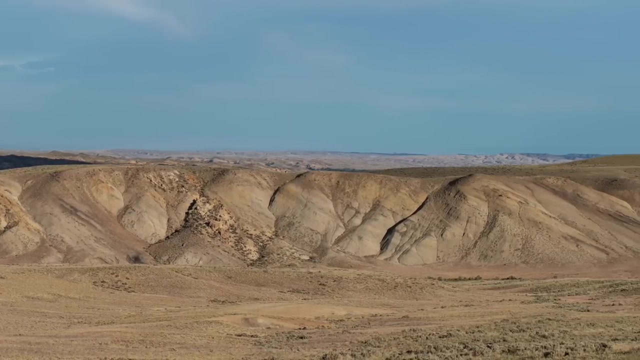 Went clear up and over the mountain Been eroded back down to this ridge line Or the top of this hill, And so notice the nature of the dip And let's continue. As we move to the right, The rocks are becoming younger and younger. 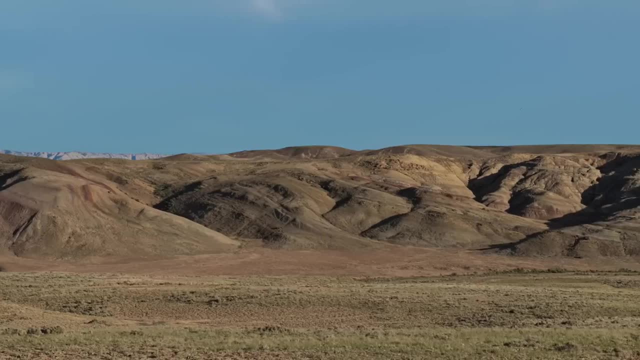 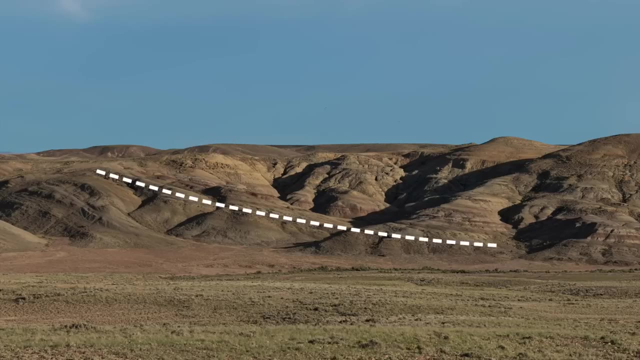 And as we move to the left, They are starting to change. They are starting to change. So I want to stop here, Because now we are starting to see Some significant change In the dip amount, Or the amount that the rock is sloped. 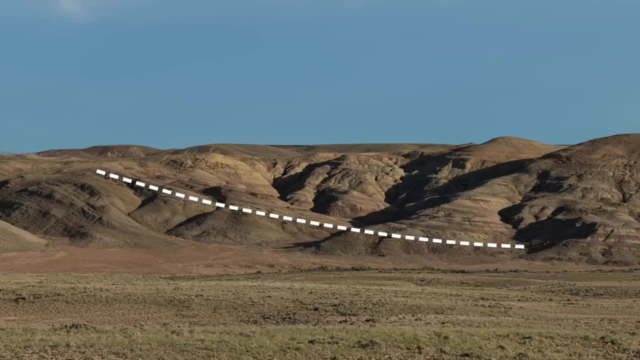 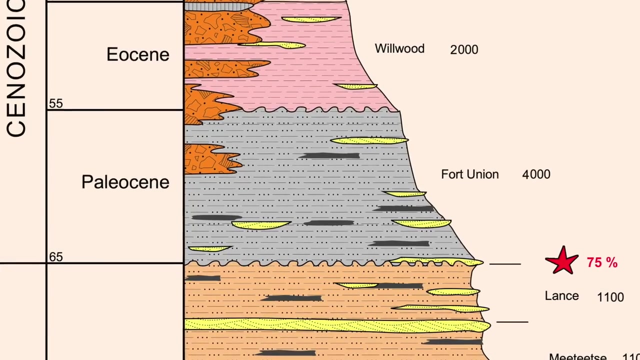 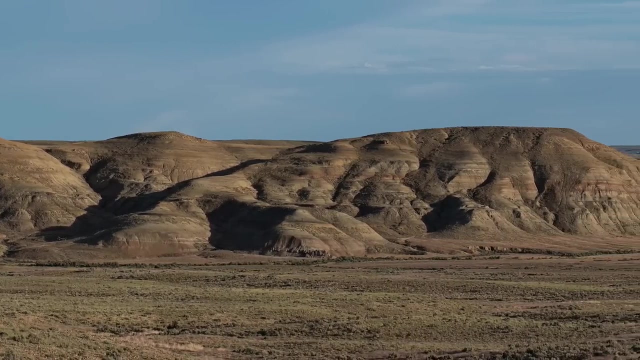 In this region. here Aren't we? It's not dipping as steeply Interesting. Another important note Is that below this white line Is the Fort Union formation And above it Is another formation, And as we approach the end of the hill, 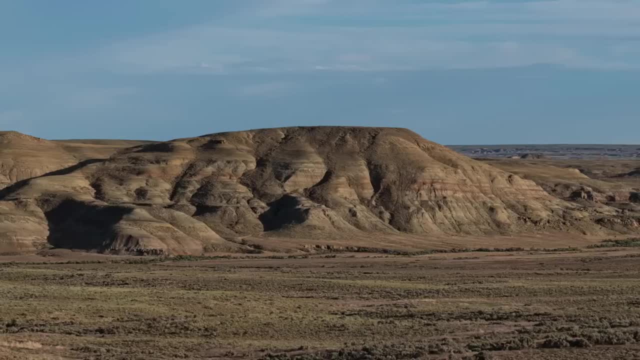 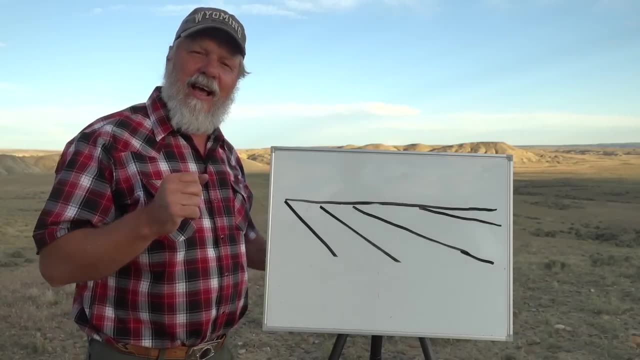 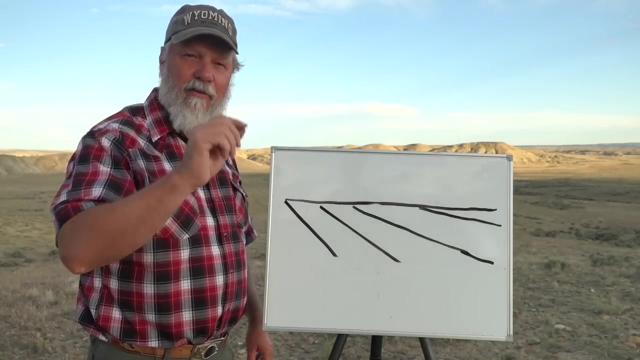 We see that the layers are nearly flat. Now that you've seen a video Of the hillside back behind me, You see these dipping layers That I've marked out for you And how they change Across the hillside Along back to my right. 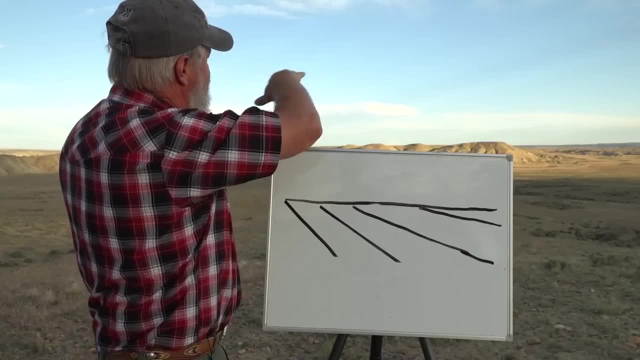 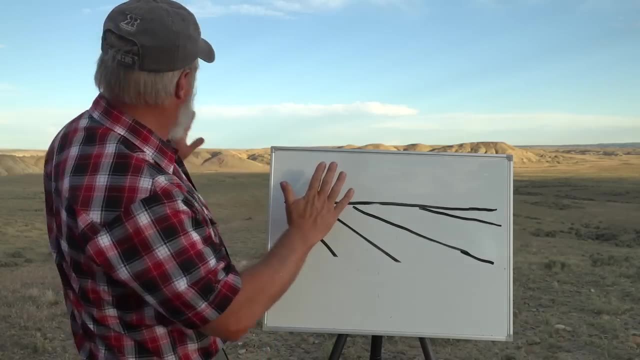 Over here right. They go from steeply dipping To flat over here to my right. So in this little drawing It's very simplified to show you that To my left, Towards the Bighorn Mountains, The beds are steeply dipping. 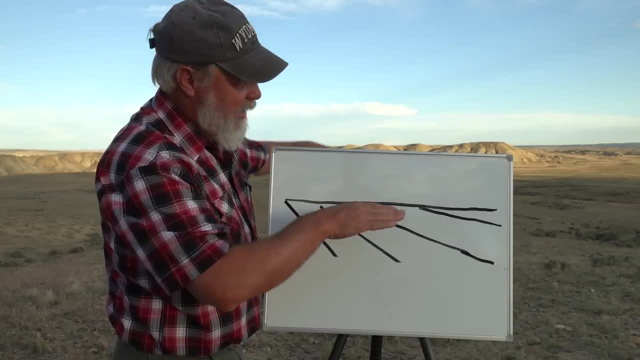 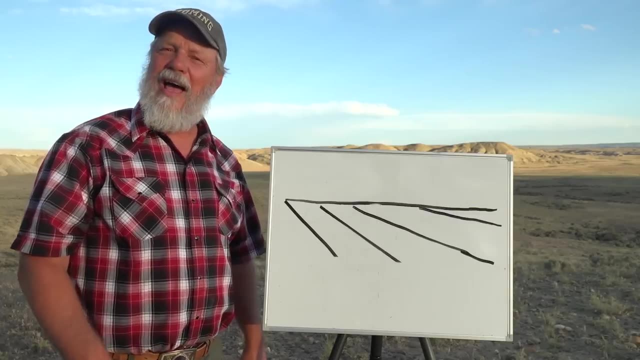 And they become flat, flat, flat. As you get out here They are getting very near flat, And as you go further into the basin They are flat. So how do we interpret What we're seeing here in the hillside? 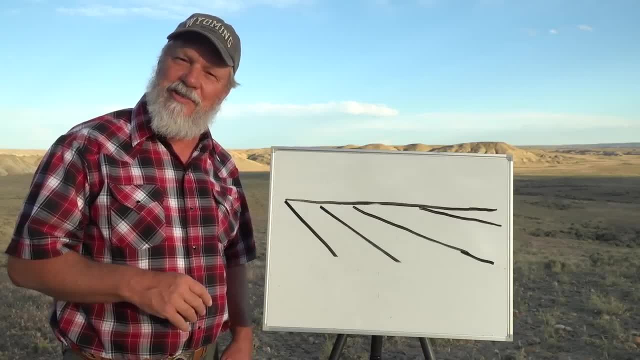 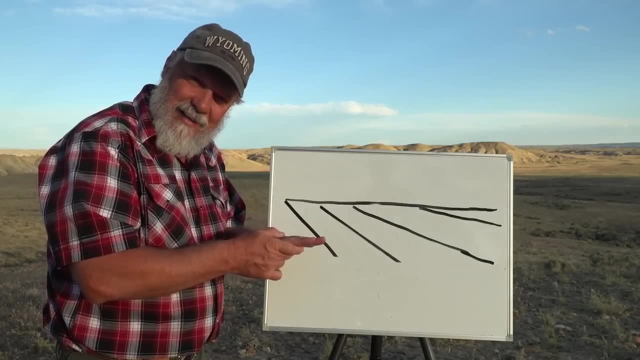 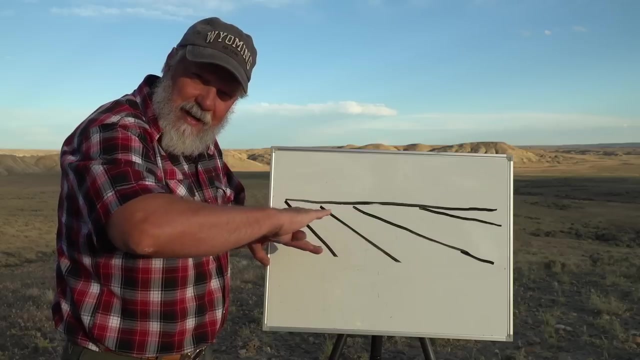 Well, we use the basic geologic principle Of original horizontality Right. So if my hand represents the original bed, This one here it was flat. The mountain uplifted And tilted it some, And then deposits were continually Being put in flat. 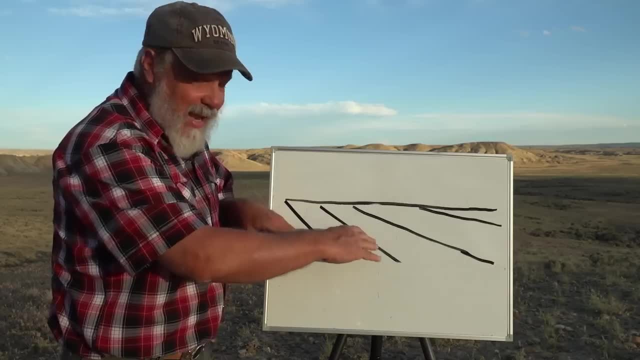 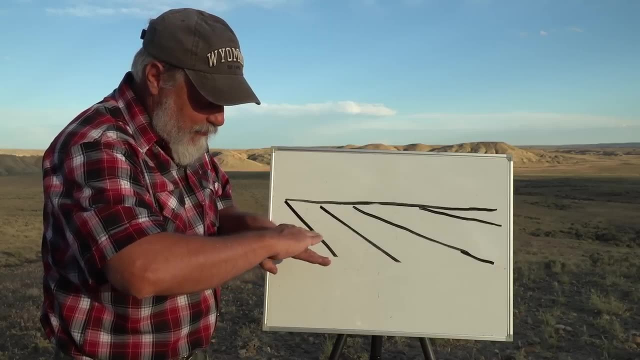 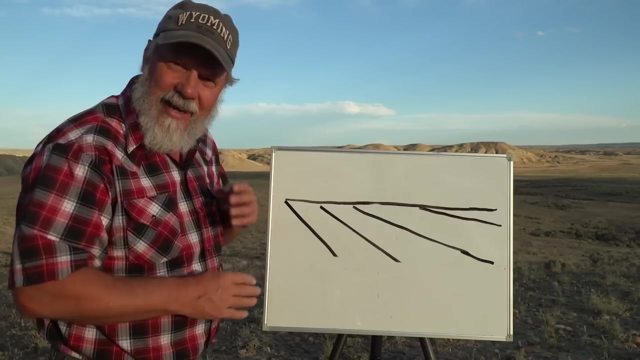 Okay, Through time, And rotated too. So this one started flat, Tilted. A new layer comes in Flat, It gets rotated. Then a new layer comes in flat, And it gets rotated, etc. But sometimes at some point. 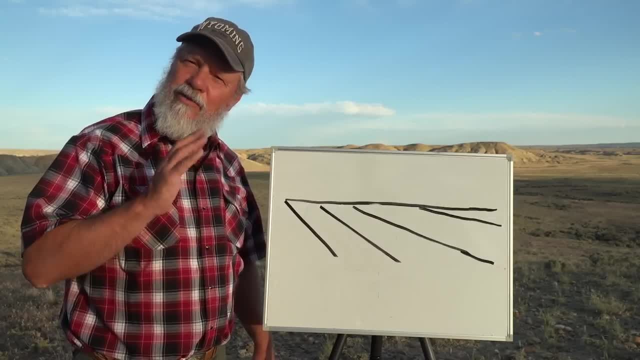 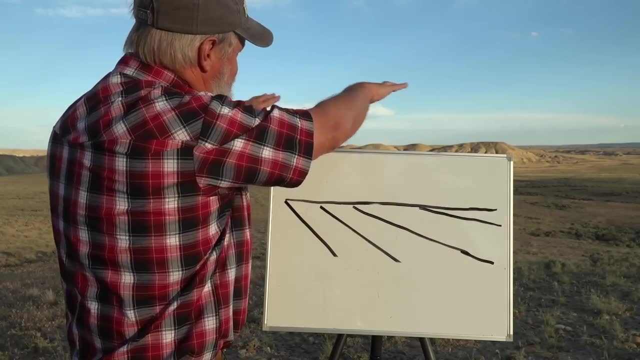 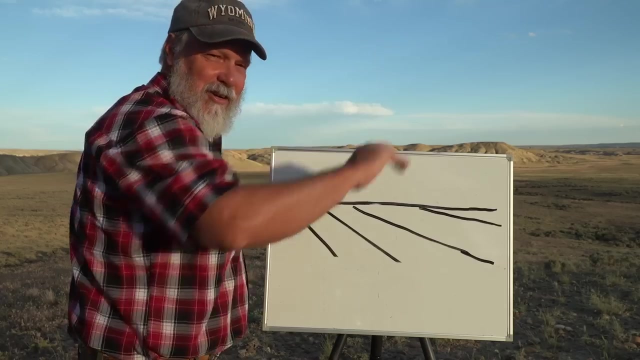 This game ends right, This deformation, The tilting stops, The mountain stops And that means that this bed here, Way out here, It was deposited And tilted just a little bit. And if you go further into the basin, This age of rock out here, 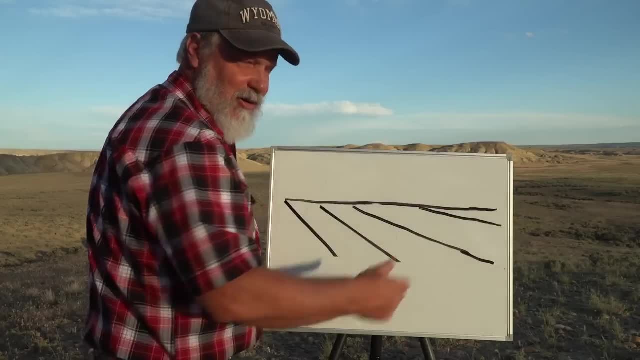 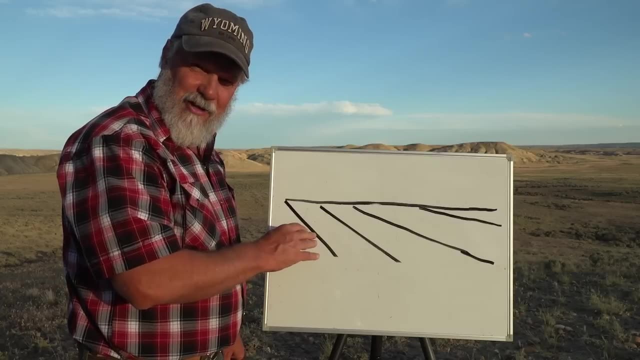 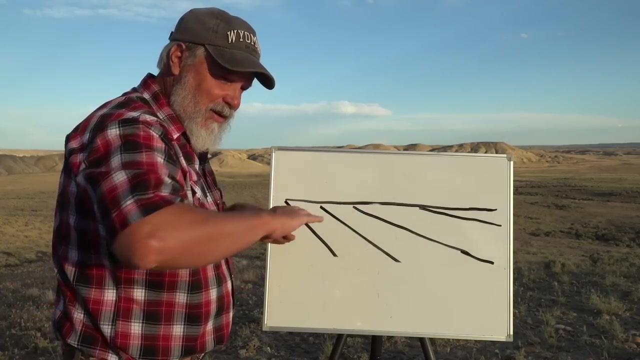 Is flat. It was not tilted As you get younger and younger. So these rocks, Where we visited the first outcrop right, Are about 65 million years old And they just keep tilting Through time And being deposited on the sides. 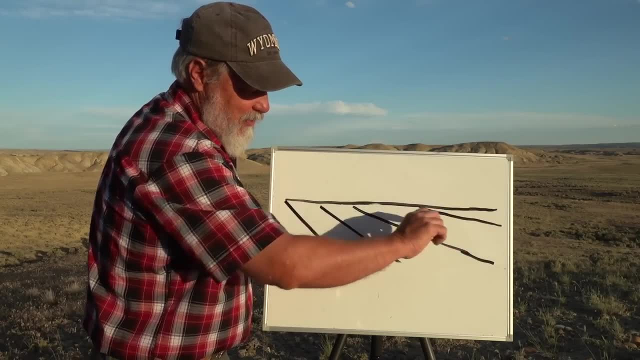 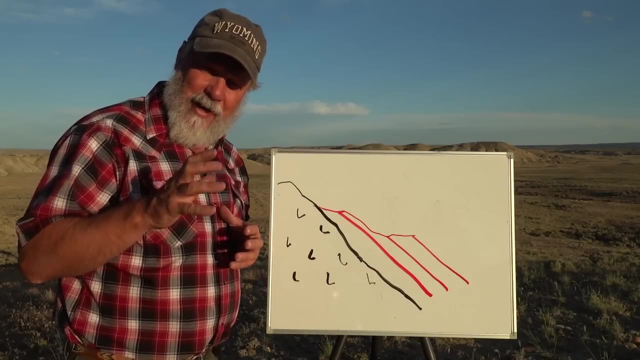 And we can date these Sediments out here, Formational layers Which I want to touch on for just a minute. So I wanted to To bring radiometric dating Back into the picture And explain that just a little more clearly. 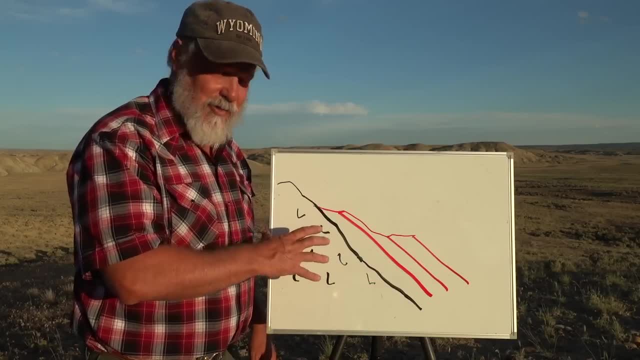 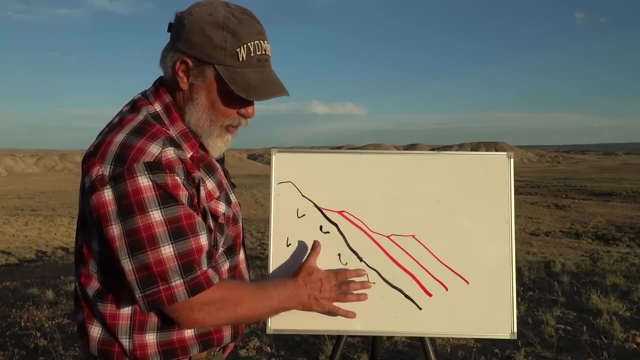 Here's a mountain here, Like we've seen in the Wind River Mountains, The Bighorn Mountains, All these mountains in the Rocky Mountains, Primarily nearly all of them are the same. They have a core of very old rock. This is crystalline rock. 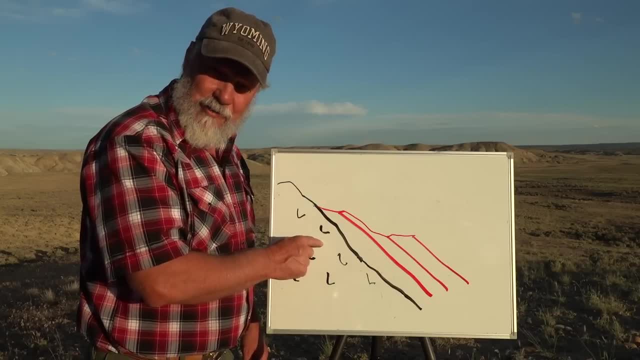 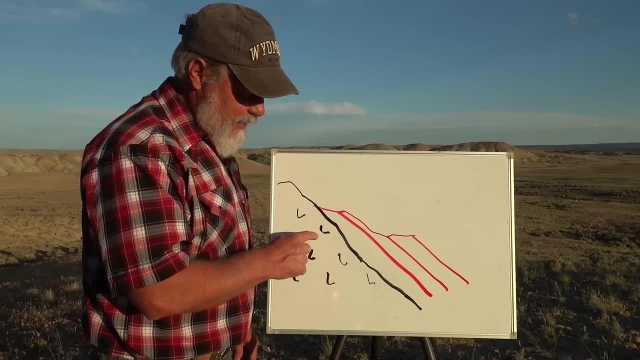 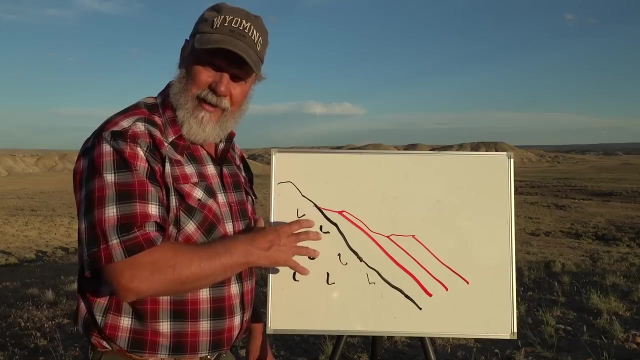 If we go in And date this radiometrically And grab a piece of that, What are we dating? We're not dating the age of the mountain. We're dating When this molten rock, This igneous rock, Once was liquid. 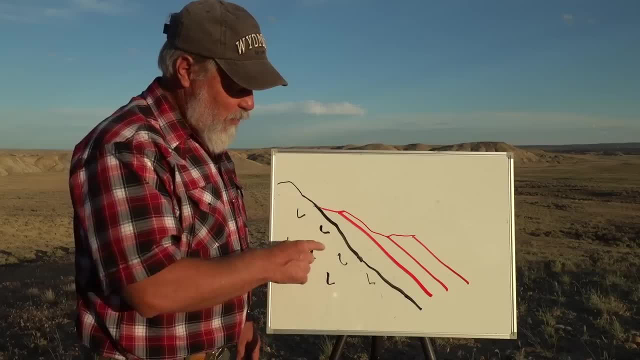 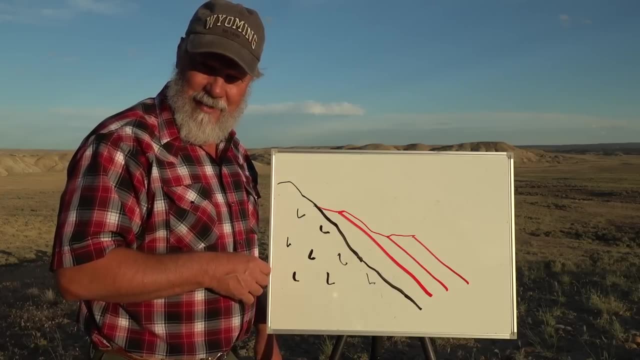 And cooled into crystals. That's what we're dating. So when we date the core of the Bighorn Mountains, We get 2.7 billion years old, Not 65 million. So, Using these principles, though, We do know. 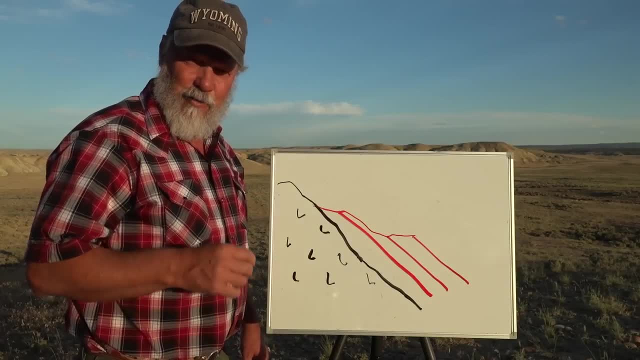 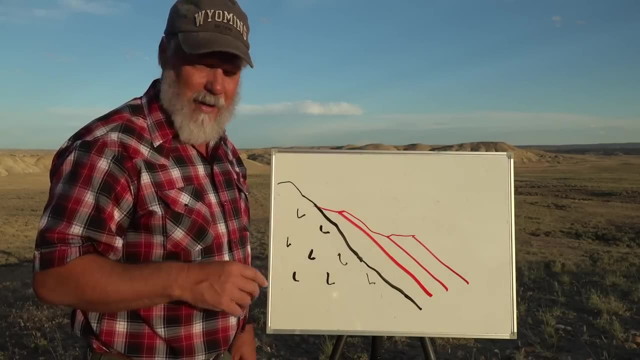 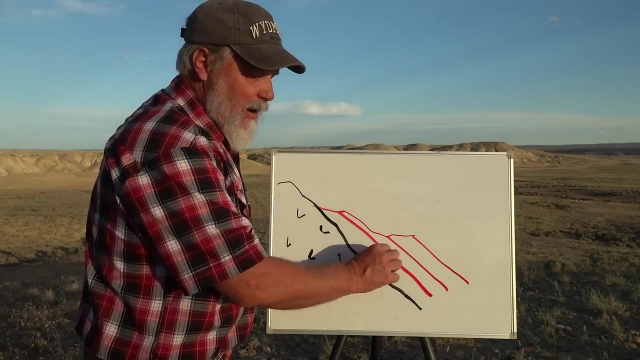 The ages of the formations And radiometric dating Is used to date those. We'll find an ash layer In one of these beds Somewhere. It could be a long way from here Because these formations go a long way. They'll cover an entire state and more. 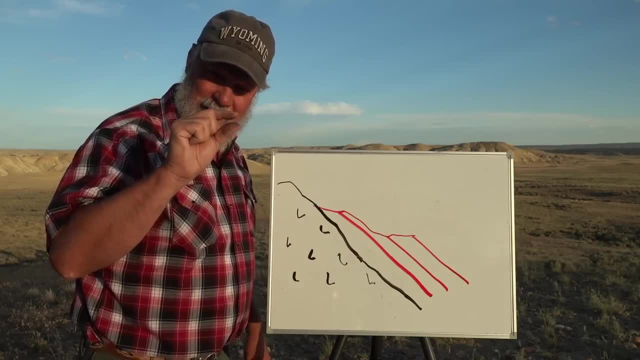 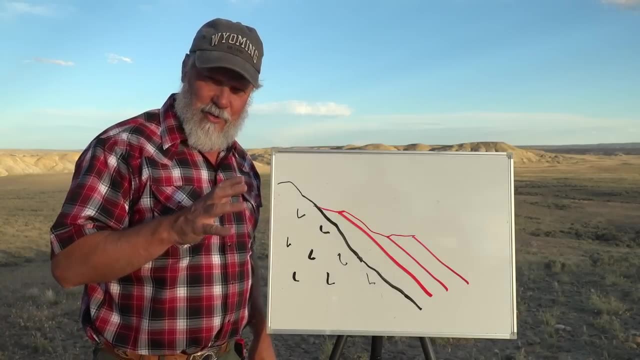 And so we find opportunities Where we'll have a deposition of volcanic ash And that is a valid date That lays in on one of these formations, This process that I've shown you. If you had no idea, If you had no radiometric dating at all, 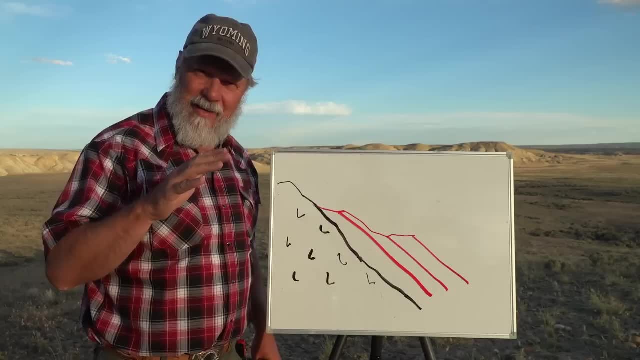 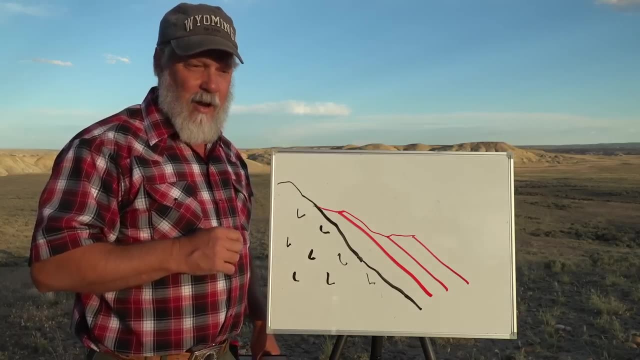 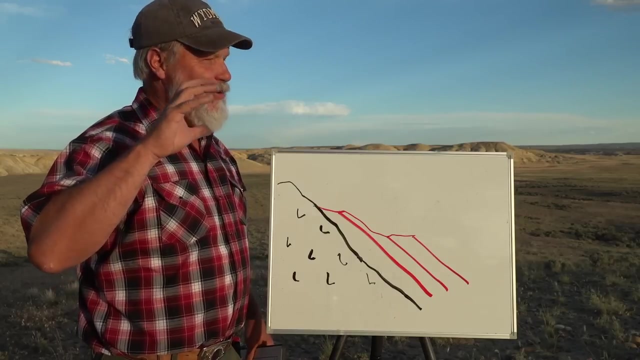 You could still know When things happened relatively. We call it relative dating. We know when it started, What formation of rock, And we know what ended. You know when it ended In a certain formation of rock, And then we use radiometric dating. 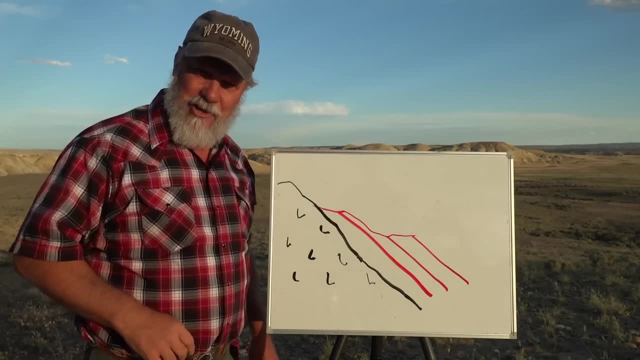 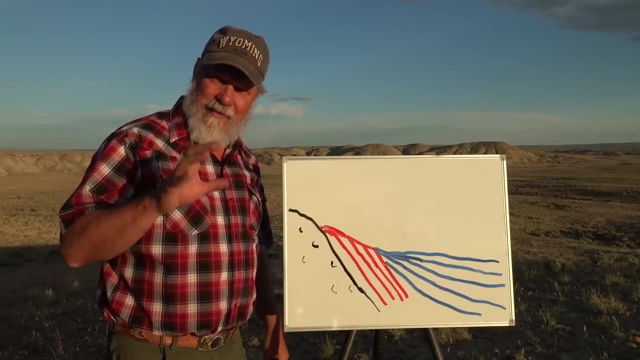 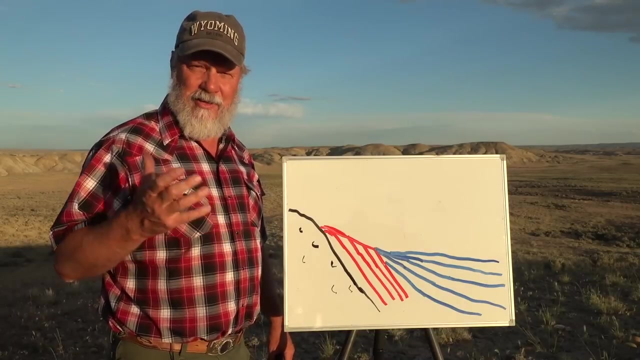 To get the absolute dates When we date those formations. So I've taken This nice outcrop That we have That information Combined with the prior stop we had, And I've sketched out the big picture Which applies to. 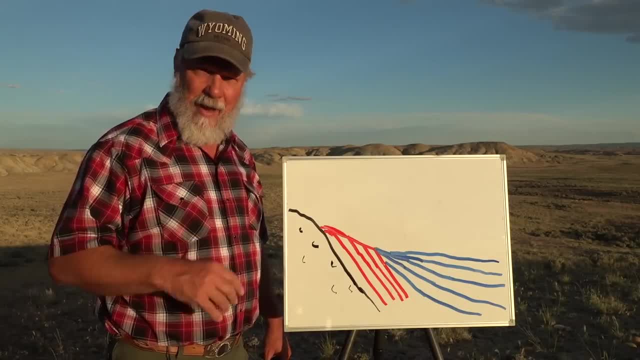 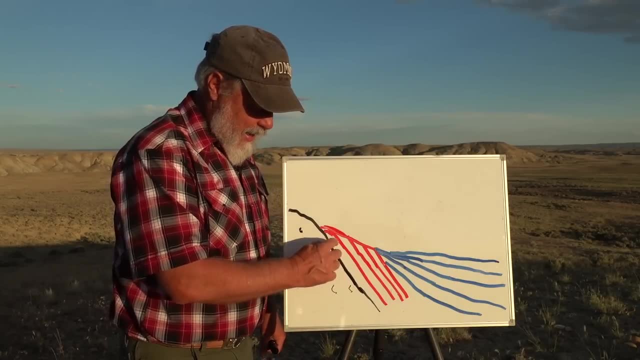 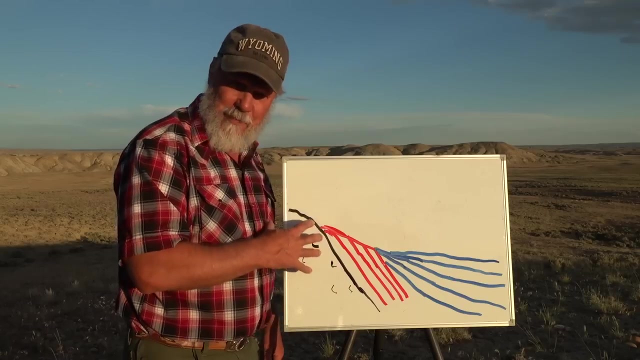 Many of the mountain ranges In the Rocky Mountains. We have the core- Very old granites And metamorphic rocks- And then we have these old rocks That were there, That were there Prior to the uplift of this mountain That I've talked about. 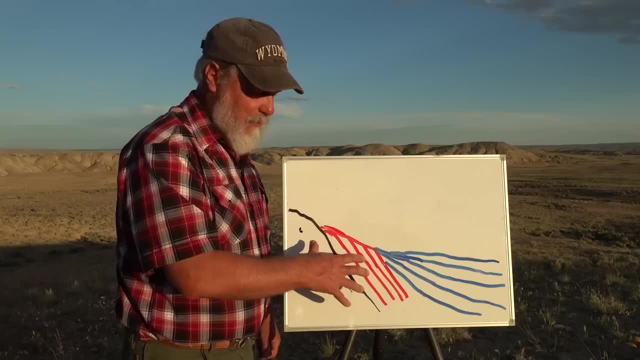 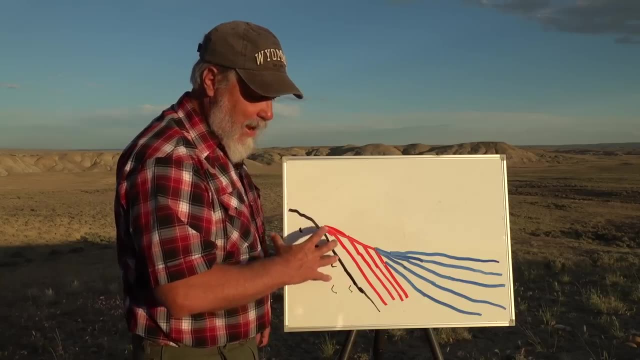 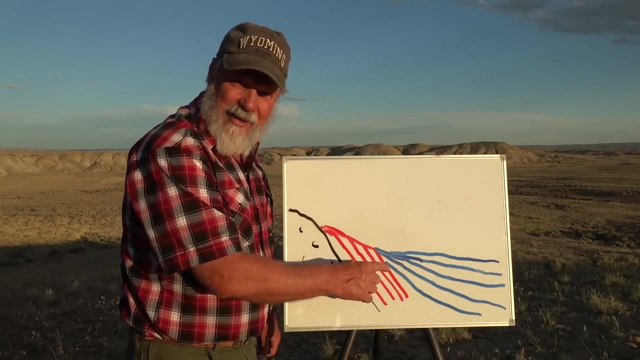 All the red- They were there prior to the uplift- And then All the blue layers of rock. The formations were being deposited As the mountain was uplifting, And that's where we've been looking At these unconformities. Our first stop was 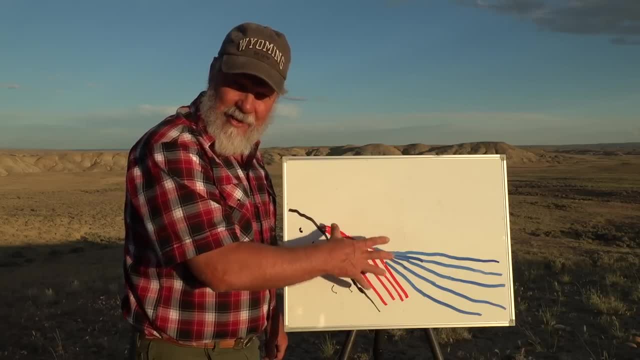 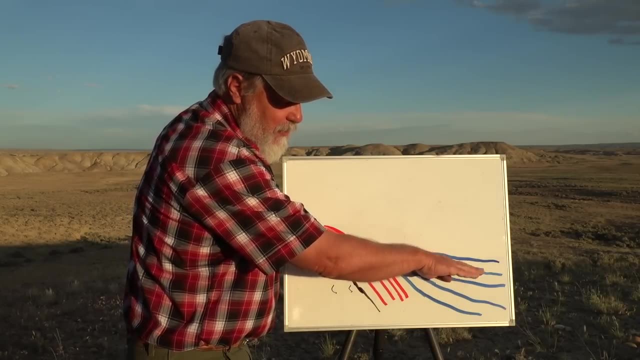 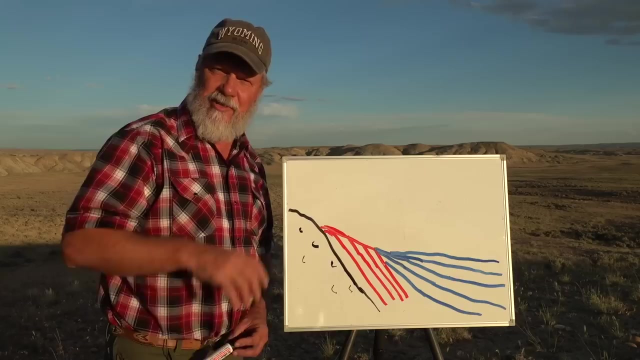 A spectacular angular unconformity In this general area, In this sketch, diagrammatically. And this stop, We're out here where things are going from Pretty steep to flat. Okay, And it tells us That's when the mountain stopped. 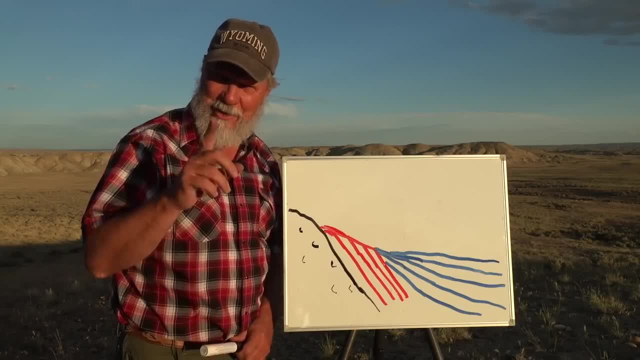 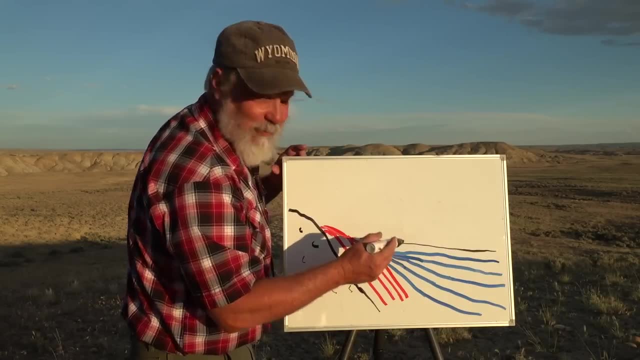 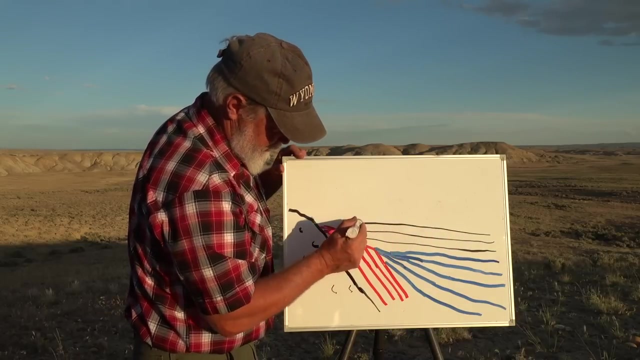 And once it stopped, An amazing thing happened. In many of the basins here, Especially in Wyoming, Is sedimentation continued to occur, Depositing flat across- Hopefully I'm drawing horizontally here Right- Just kept filling in The entire basin out here. 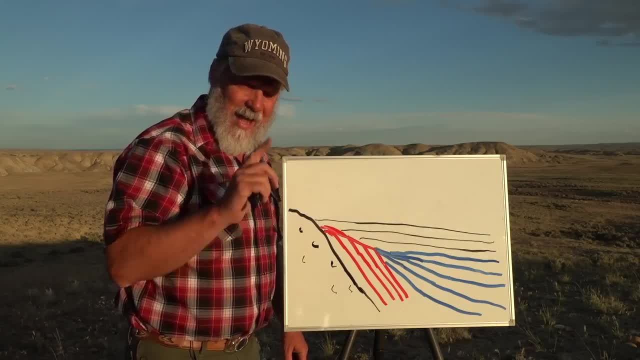 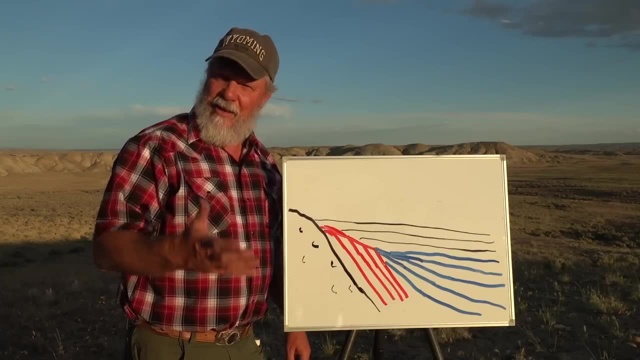 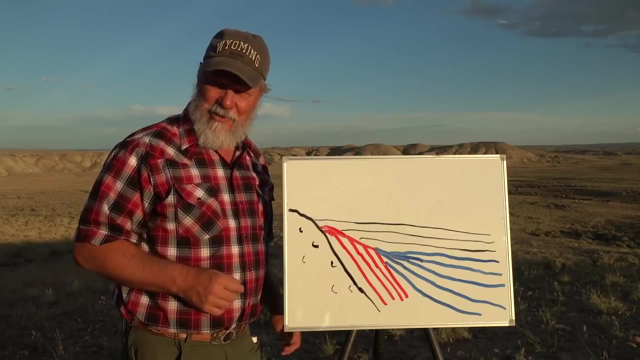 Right up To nearly the tops of the mountains, To the very peaks, Because the story of that Is really amazing In my view. So I think you see That using very simple geologic principles, We can unravel amazing history And determine.